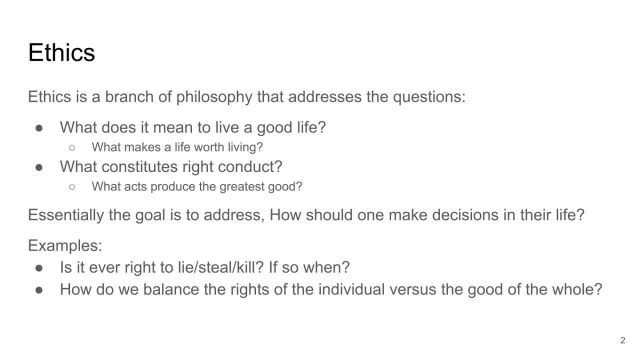 harm an individual if there's going to be a greater good. And I think that oftentimes when we teach engineers, we like to focus on these broader topics because they're actually very interesting. We like to tell engineers: say, you're working for a company that's making self-driving vehicles, How do you know when it's right to swerve into? 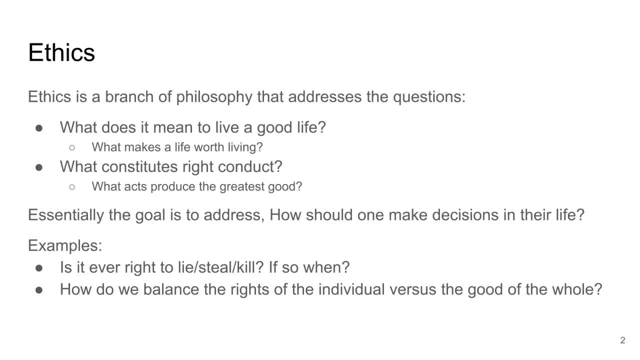 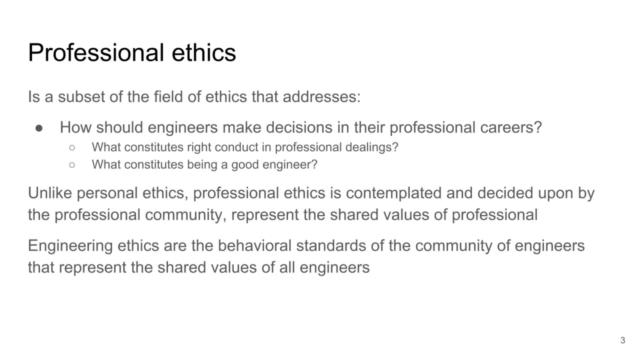 the sidewalk? How do you balance the safety of pedestrians and the safety of the driver? And I think that those are important questions and those are questions that each individual has to address, but that's not necessarily what professional ethics is about. Professional ethics is a subfield of ethics in which we talk about how, within a certain 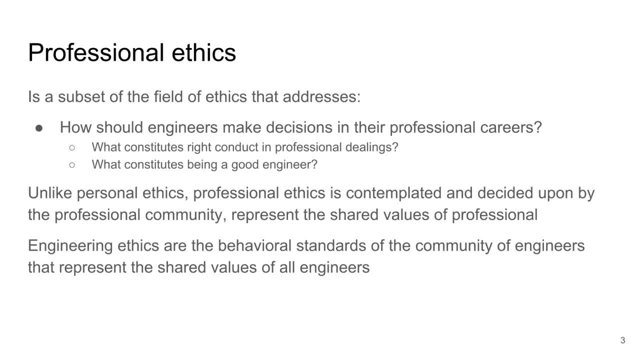 profession. you should behave So as an engineer. we say: how do you make decisions as a professional? that makes you a good engineer? What constitutes a successful, right conduct as an engineer? something that's different about professional ethics versus individual ethics is that it is a set of values that are decided upon by the professional. 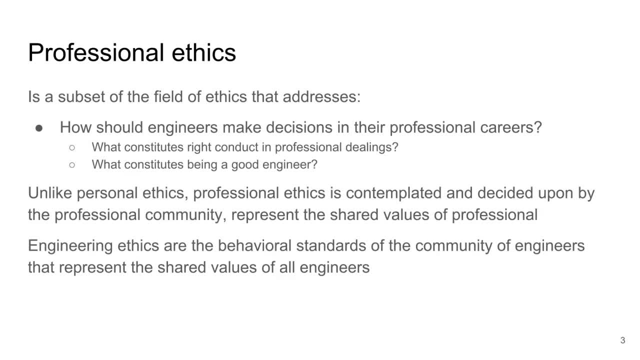 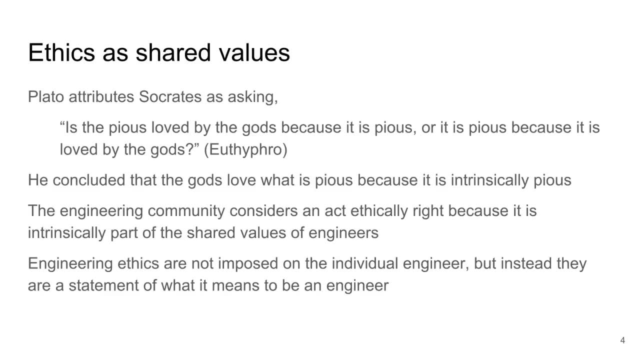 community, and these are shared values that all engineers have. So Plato wrote- and he attributed this to Socrates- that you know, is the pious loved by the gods because it is pious or is it pious because it is loved by the gods? so, is an act good because God said it's good or is an act good? 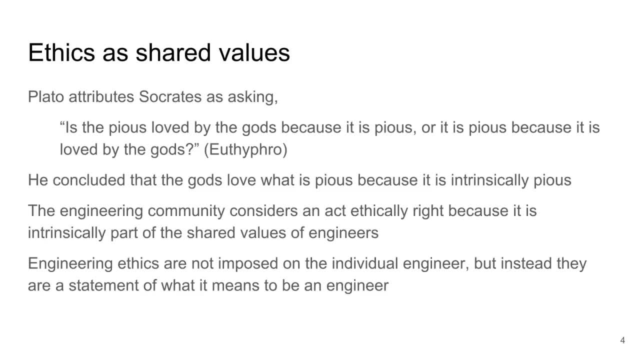 therefore, God said it's good, says is good, And he concludes that certain actions, certain things are intrinsically good and therefore God loves those. And I think when we teach engineers about ethics, we oftentimes say: well, we have these ethical standards and you have to live up to those because they're important. 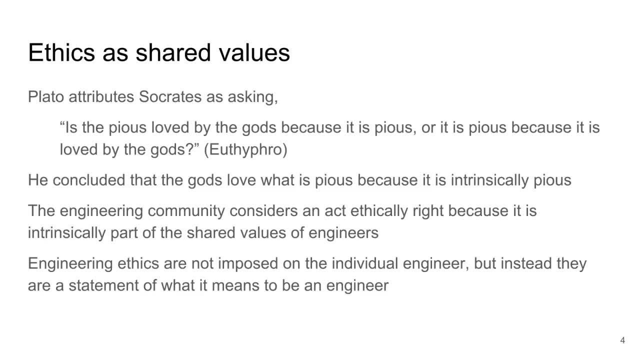 for the community, they're important for public safety, But I think that it's actually a bit backwards And these ethics that engineers have are not externally imposed. Say you must do this because there's going to be some good outcome, But instead these are intrinsically shared values. 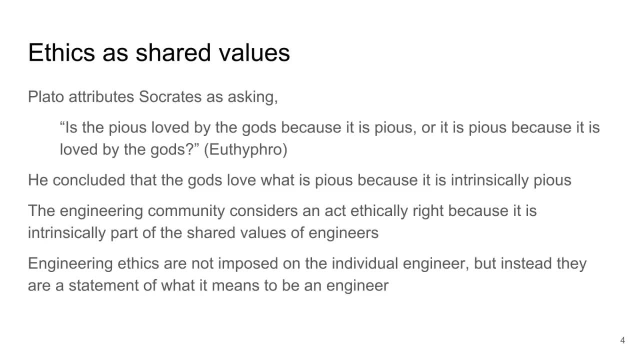 of engineers and they're intrinsically good and make good engineers, And I think that's also something that in the teaching of engineering ethics people get wrong- That these shared values already exist, And what we're essentially doing here is we are listing these and clarifying them. 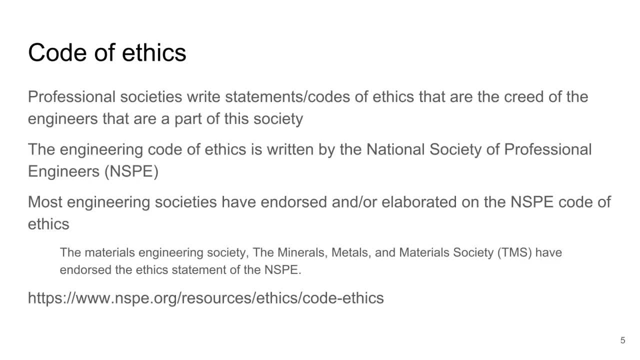 So we wind up with these code of ethics that have been written by our professional societies, And these code of ethics are, as I said, not externally imposed, but they're just a statement of what we, as engineers, believe. The most common one, I would say, is the code of ethics written by the National Society of 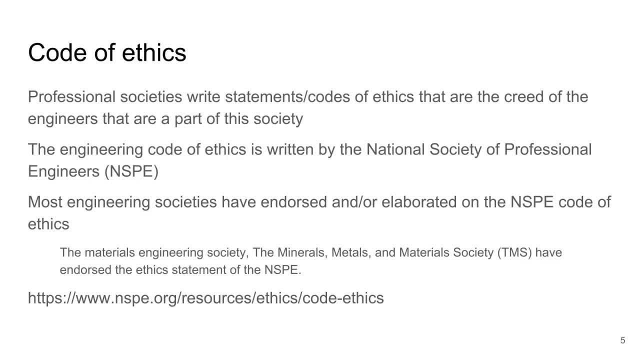 Professional Engineers, And that's what I'm going to be talking about today- But most engineering societies, whether it's material science or mechanical or civil, those societies have either endorsed the NSPE code or they've endorsed the code of ethics, And so I think that's a statement of 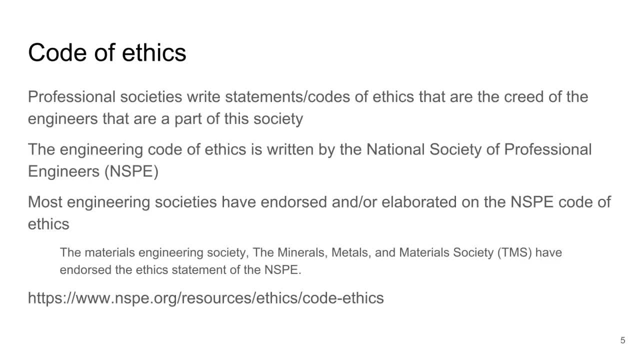 ethics, that they've endorsed it and modified it in some sense. In the case of material science, which I am a part of, the Minerals, Metals and Materials Society, TMS, they've endorsed the ethics statement of NSPE, And those are then the same ethics that materials engineers are expected. 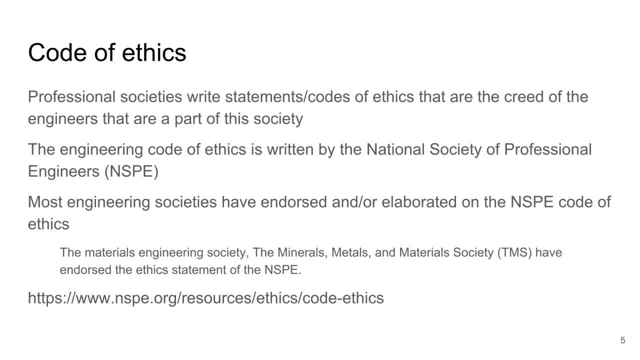 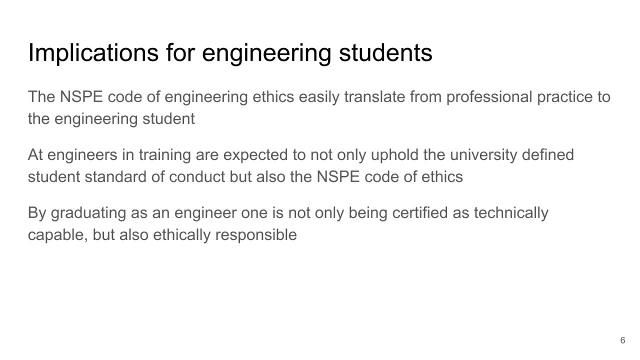 to conduct themselves by. So I've put a website on the bottom of this page where you can look up these code of ethics, and I'm going to be talking about those in this lecture. So the implications of this code of ethics for engineering students is that students are expected. 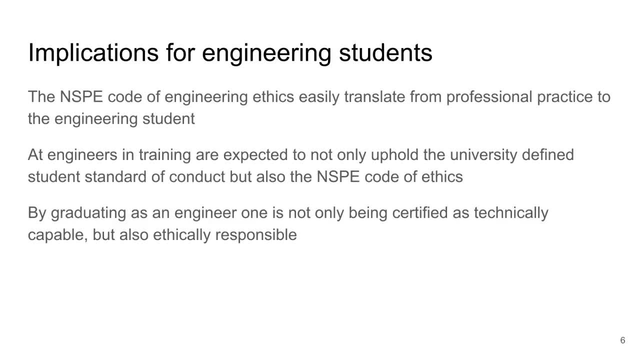 to learn and internalize these ethics as they study to become an engineer. So engineering students are expected to not only uphold their university's code of conduct and honor code, but also the code put forward by the NSPE. And of course it's a learning process, so mistakes will be made And as faculty we step in and try to write things. 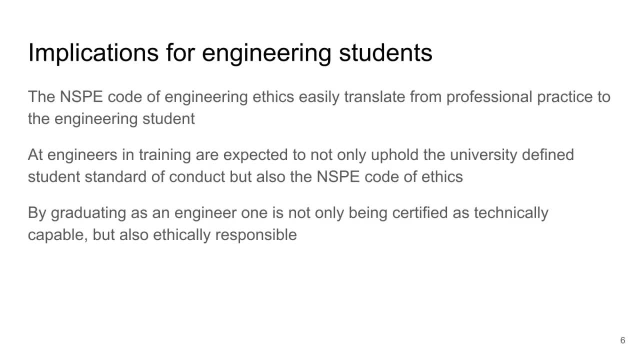 But the important thing is that when a student graduates as an engineer, they're being certified not only to be technically capable, but also that they understand the values and obligations of being an engineer. So I'm going to go through the NSPE code of ethics. 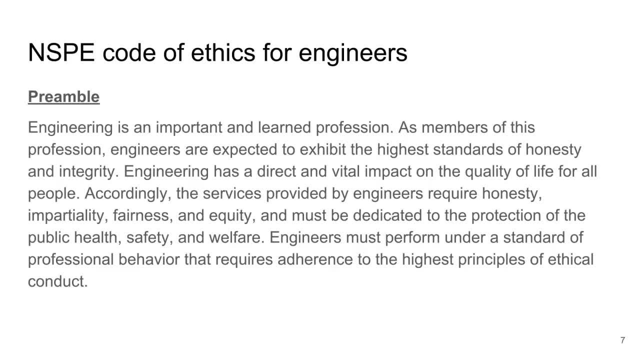 Beginning with the preamble. So the preamble reads: engineering is an important and learned profession. As members of this profession, engineers are expected to exhibit the highest standards of honesty and integrity. Engineering has a direct and vital impact on the quality of life for all people. Accordingly, the services provided by engineers require honesty and 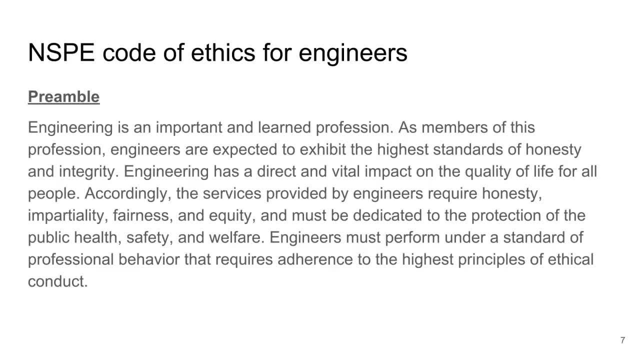 impartiality, fairness and equity, and must be dedicated to the protection of the public- health, safety and welfare, And engineers must perform under a standard of professional behavior that requires adherence to the highest principles of ethical conduct. So this is a statement. You think of it as the pre emblem to the creed of engineers, And it talks about 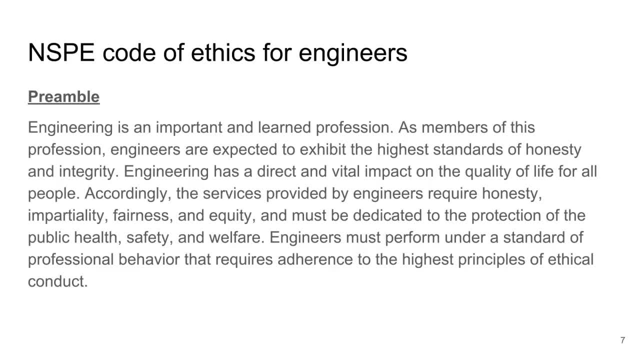 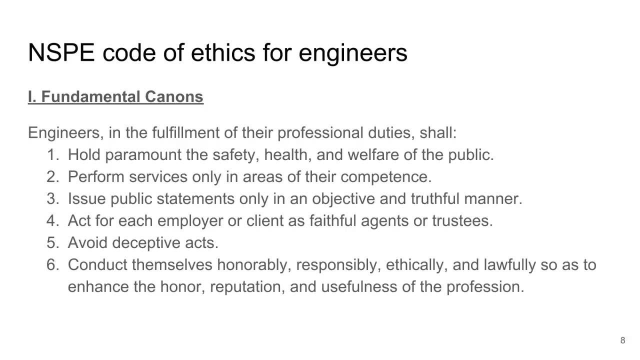 engineering as its importance and its role in society and why, as engineers, we hold these values. After the pre emblem, then, there are a set of fundamental canons. So these fundamental canons are that engineers, in the fulfillment of their professional duties, shall one hold. 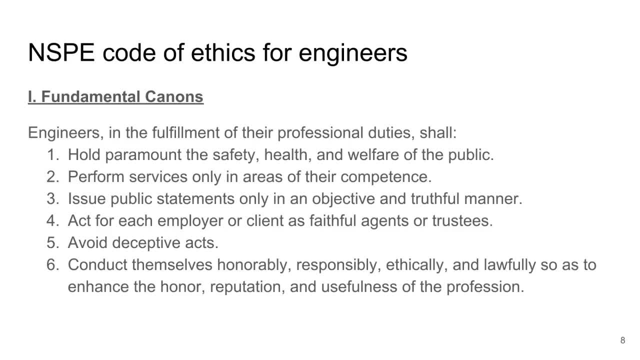 paramount the safety, health and welfare of the public, to perform service only in areas of their competence. Three: issue public statements only in an objective and truthful manner for act for each employer or client as faithful agents or trustees. Five: Avoid deceptive acts. and six: conduct themselves honorably, responsibly, ethically and lawfully so as to enhance the honor. 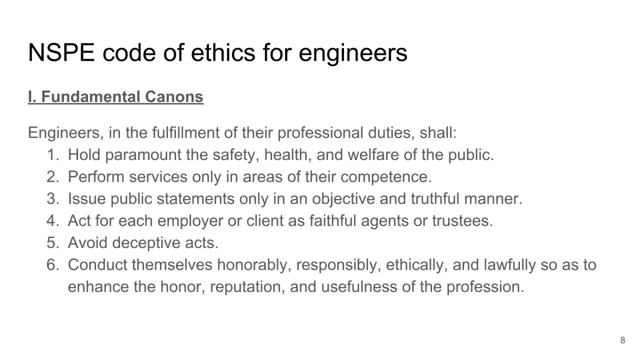 reputation and usefulness of the profession. So these canons tell us about the values that we have and about our- really our- primary targets. So we have a duty to ourselves. Of course, that's all. people have a duty to themselves, But we also have a duty to the public. 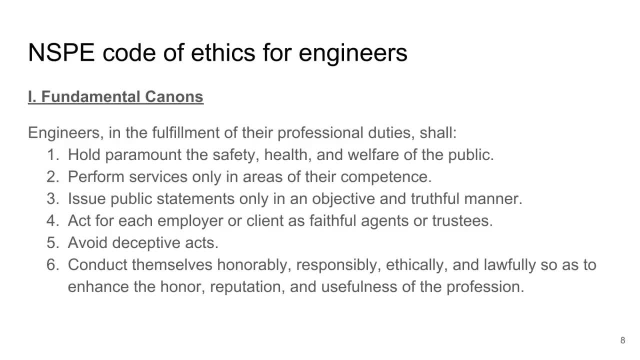 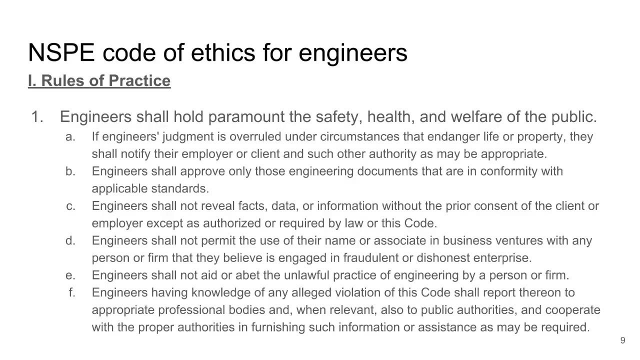 We have a duty to our employers or clients and we have a duty to the greater engineering community to generate honor, reputation and respect for all of engineers. So, following the canons, we have a set of rule of practices, And I'll read through these and talk about these. 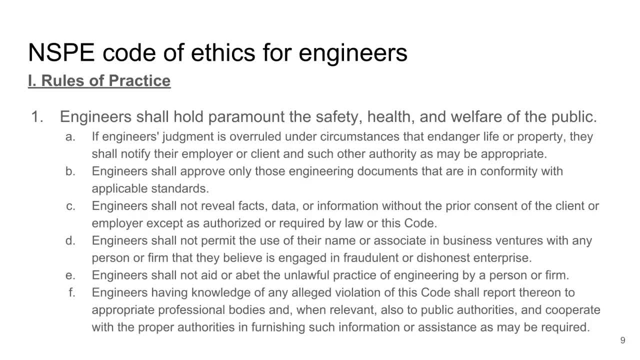 So first rule of practice: engineers shall hold paramount the safe health and welfare of the public. A if engineers judgment is overruled under circumstances that endanger life or property, they shall notify their employer or client and such other authority as may be appropriate. So this is saying that as an engineer, you work for an employer. 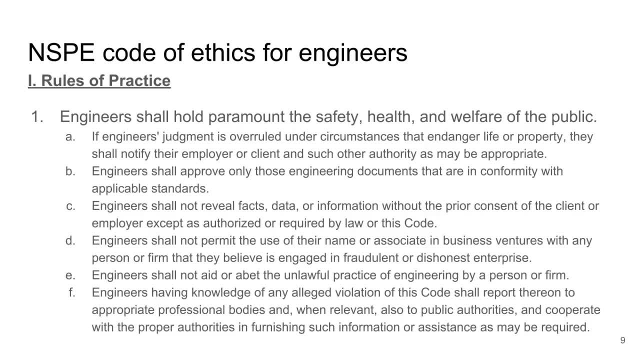 But if someone overrides your judgment And you think that this endangers the health and welfare of the public, you have a responsibility to you know, move up the administrative chain in your company or even go to an outside source or an outside authority to report where there may be danger for the public. 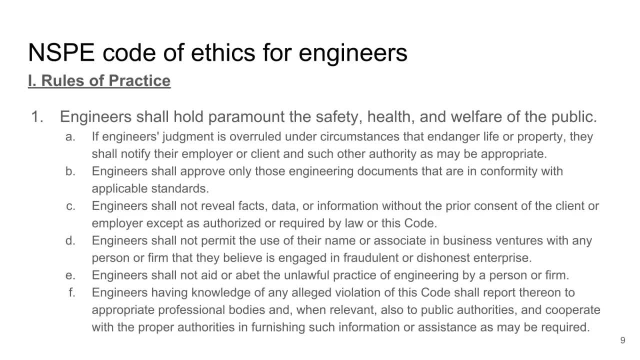 B, engineers shall approve only those engineering documents that are in conformity with applicable standards. So, engineers, we have a set of rules. So, engineers, we have a set of rules. So, engineers, we have a set of standards for our, for our decisions. 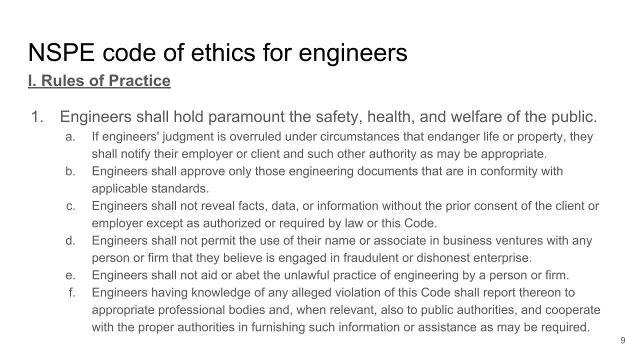 These standards have been written out by our professional societies that tell us, for example, how is it appropriate to test a certain situation? How is it appropriate to, for example, say you're measuring the strength of concrete? There is a standard for how you measure the strength of concrete. 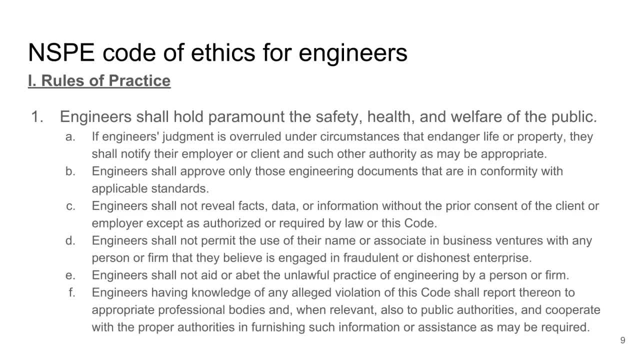 And we are, And we are required to understand what these standards are and to apply those. so that's part of how we make decisions about what is safe for the public. you know, if you have, say, an employer and you're measuring the strength of concrete and your employers, well, I know what the standards are, but I want you to do something else. 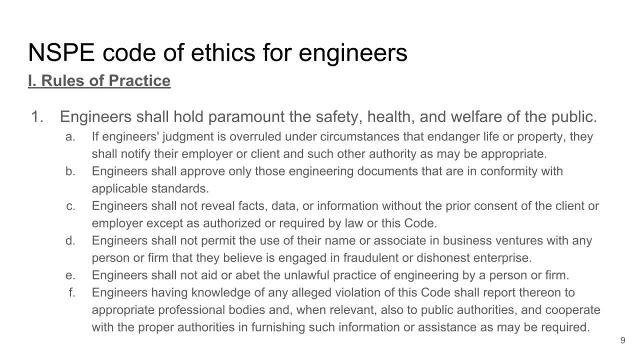 Well, you've just come to a point where your ethics are being questioned because you're being asked to apply standards or apply a measurement which is not applicable. Well, you've just come to a point where your ethics are being questioned because you're being asked to apply standards or apply a measurement which is not applicable. 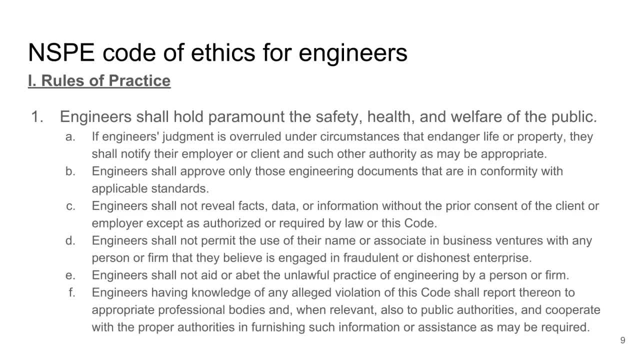 Well, you've just come to a point where your ethics are being questioned because you're being asked to apply standards or apply a measurement which is not applicable. So in this document, when we talk about standards, we're not talking about just arbitrary standards. 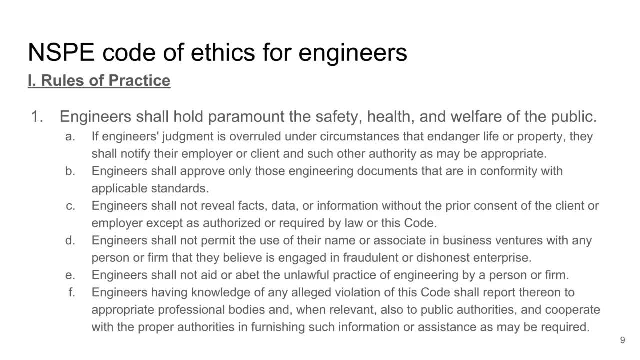 We're talking about standards that have been approved by our professional societies. See, engineers should not reveal facts, data or information without the prior consent of the client or employer, except as authorized or required by law or this code. So, even though you are required to whistleblow if your employer or client is, 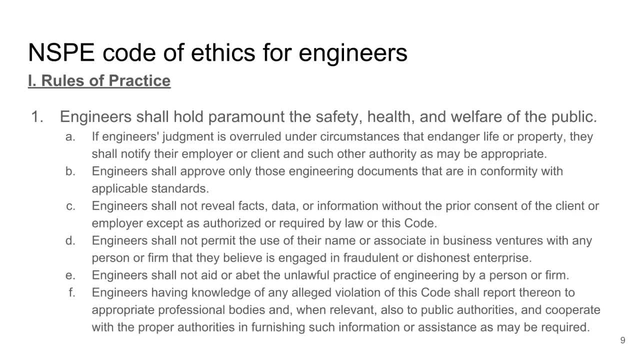 Endangering the public. if they're not, then you're required to not reveal any information about the product or the job you're doing. D engineers shall not permit the use of their name or associate in business ventures with any person or firm that they believe is engaged in fraudulent or dishonest enterprises. 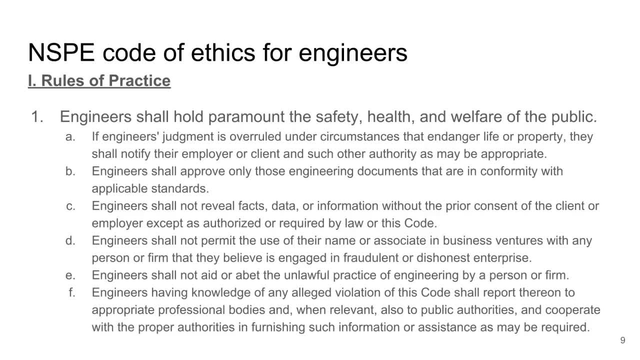 So again, this is about protecting both yourself and the name of engineers, Because you're not allowed to endorse enterprises that you believe are endangering the public or are defrauding the public. E engineers shall not aid or abet the unlawful practice of engineering by a person or a firm. 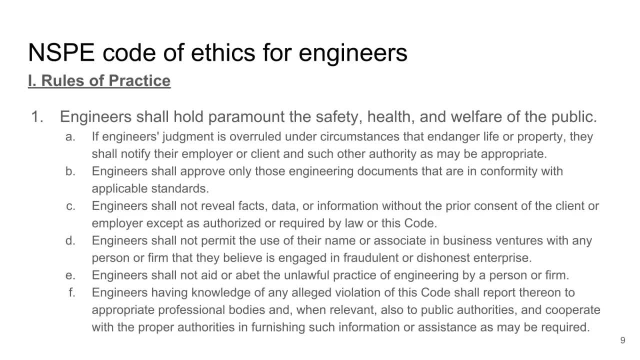 So unlawful practice. that's in part about laws and it's also in part about engineering standards. For example, professional engineers are Licensed, so companies and individuals, They have to be licensed by the National Society of Professional Engineers and going outside of that, 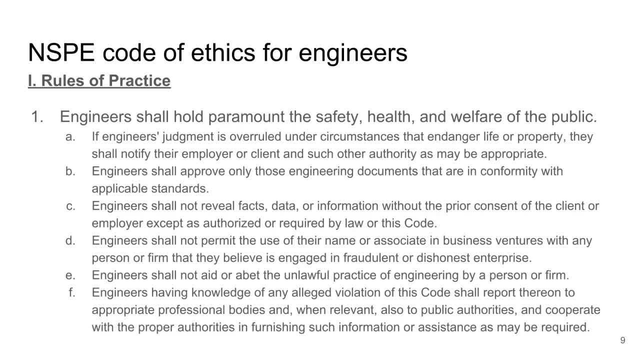 Is unlawful. F engineers have knowledge or any alleged violation of this code, shall report there on to the appropriate professional bodies and, When relevant, also to public authorities, And cooperate with the proper authorities In Furnishing Such Information Or assistance as may be required. 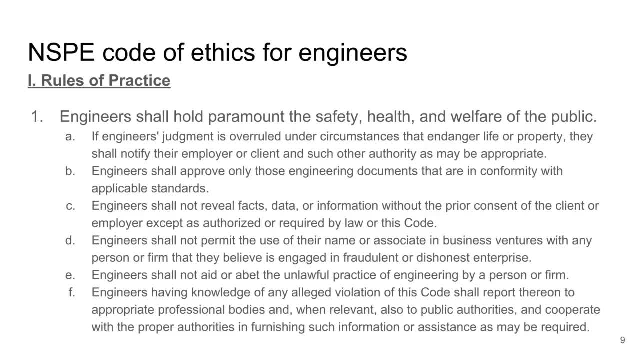 So this is telling you how to act when you believe that the safe, safe, healthy and welfare of the public or any other form of this code and violated. It's important that we have this because it gives us a process by which to investigate possible code violations, ethics violations and 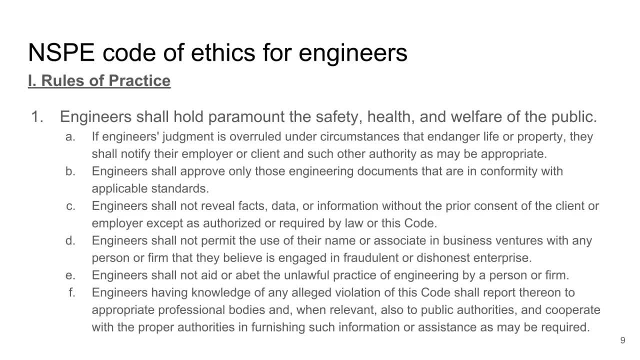 It. It avoids the situation where, for example, we have mob rule or we have people being Guilty by accusation. You can have an accusation, but then we have a set of Processes by which that these are investigated, And the National Society of professional engineers is one of that, but also just the different professional bodies. 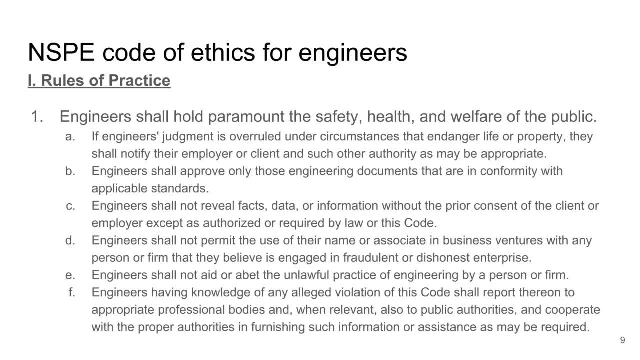 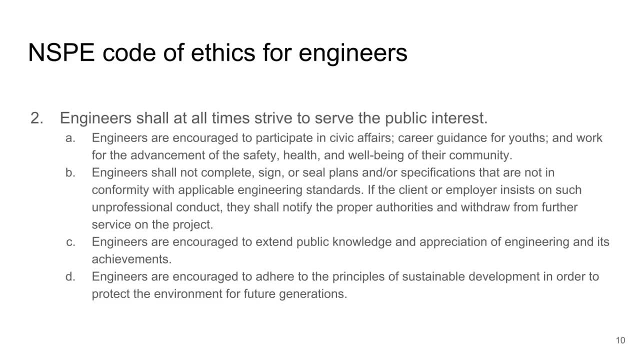 Of, For example, Tms for materials engineers. Point two: engineers should at all times strive to serve the public interests. Point A: engineers are encouraged to participate in civic affairs, career guidance for youths and work for the advancement. safety, health. 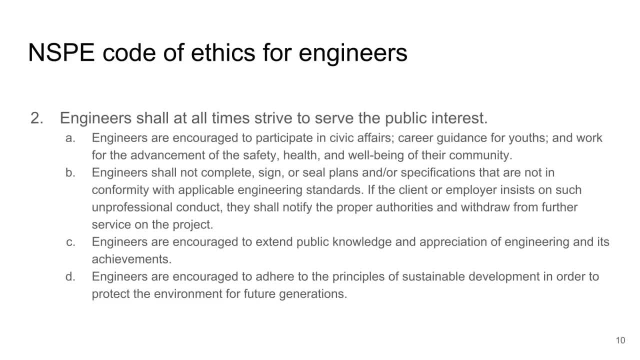 and well-being of their community. So you're encouraged to engage the public as engineers. B engineers shall not complete, sign or seal plans and or specifications that are not in conformity with applicable engineering standards If client or employer insists on such unprofessional conduct. 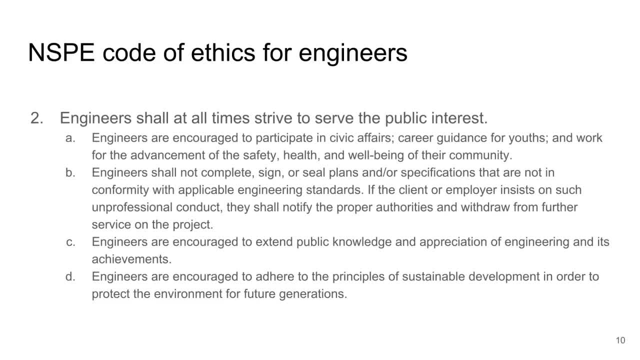 they shall notify the proper authorities and withdraw from further service on this project. And we discussed that. We have standards and if someone wants you to move outside of those professional standards then you need to alert those that are our appropriate authorities. C Thank you. 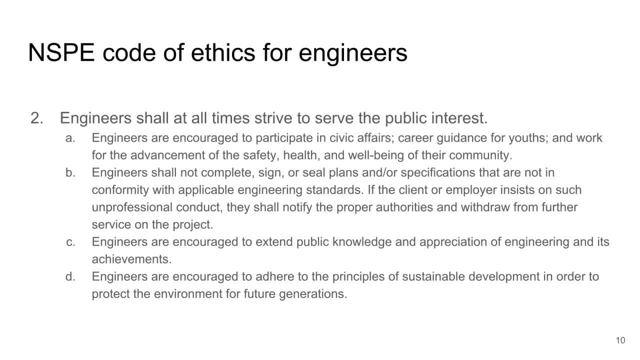 engineers are encouraged to extend public knowledge and appreciation of engineering and its achievements. so you're encouraged again to engage the public. d engineers are encouraged to adhere to the principles of sustainable development in order to protect the environment for future generations. and this is also part of, you know, looking out for the long-term public. 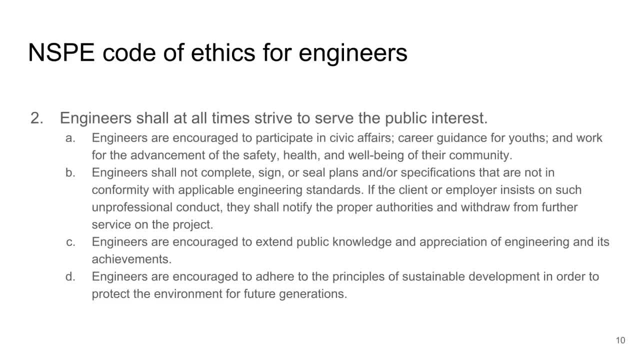 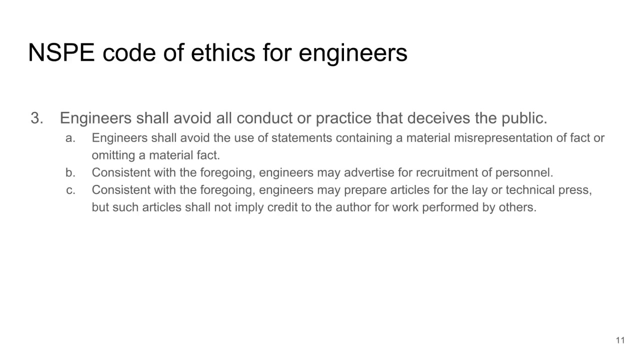 interest health, welfare and safety in the short term. many times there are big bonuses for unsustainable development, but we're, as engineers are, looking in the long term for the overall health and well-being of society. point three: engineers shall avoid all conduct or practice that deceives the public. point a: engineers shall avoid the use of statements. 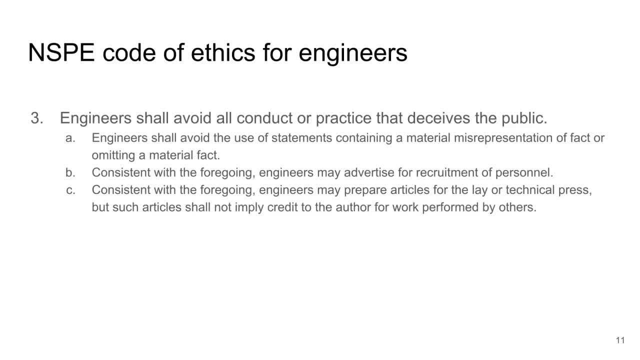 containing a material misrepresentation of fact or omitting a material fact. so when you work with the public, be honest. and if you know, for example, you're working on a pharmaceutical product and this pharmaceutical product, you know there's a material fact that, oh yeah, and it causes, you know, a rash, or oh yeah, you know, long-term exposure can cause problems. 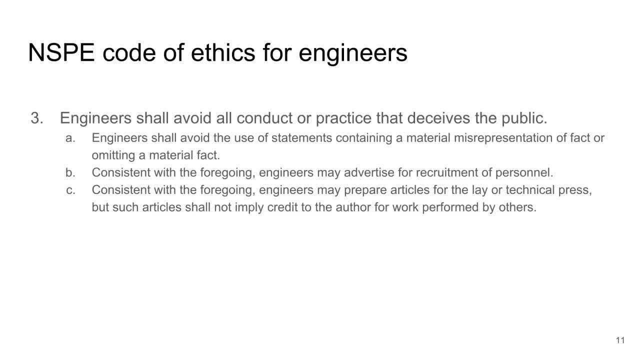 well, that has to be disclosed. whether it's disclosed, you know, through your company's legal statements, or is disclosed you know in some other fashion, it has to be disclosed. and so, honestly, i'm just saying that what i'm saying is about honesty, and it's about honesty and not about 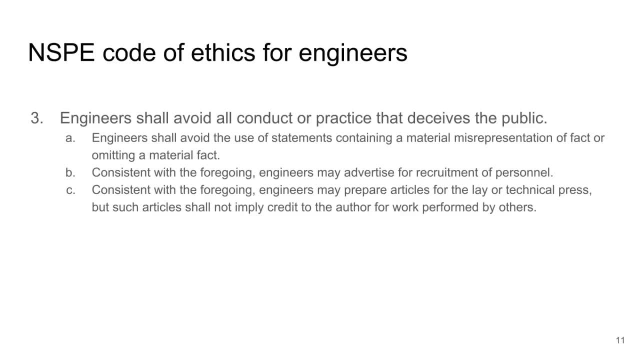 honesty, and it's not just about honesty of what you say, but it's also about honesty of what you don't say. you can't omit the facts that are important. point b: consistent with the foregoing: engineers may advertise for recruitment of personnel. point c: consistent with the foregoing. 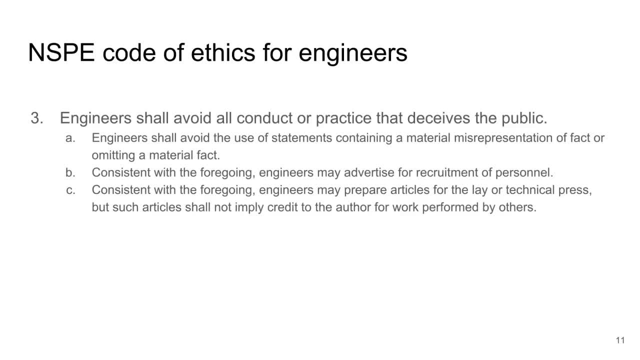 engineers may prepare articles for the lay or technical press, but such articles may not imply credit for the author of work performed by others. okay, so here we're just saying that, that maintaining this honesty about telling the truth and not omitting important content either. you can be engaged in recruitment of personnel for your companies or your clients, and you may prepare. 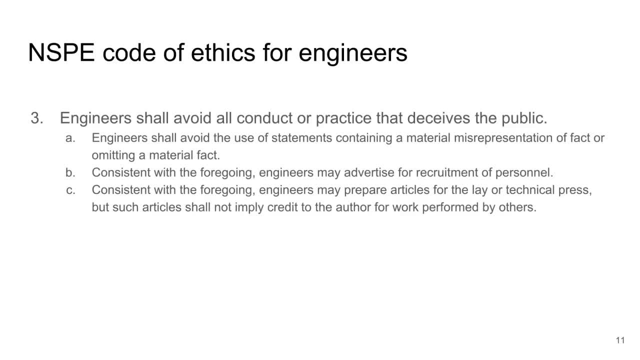 documents or, you know, video or press releases for the public, but make certain that you're being honest. and also we have to talk here about, uh, not applying credit to the author for works performed by others, so you're not allowed to plagiarize. and plagiarizing is not just about the things you've. 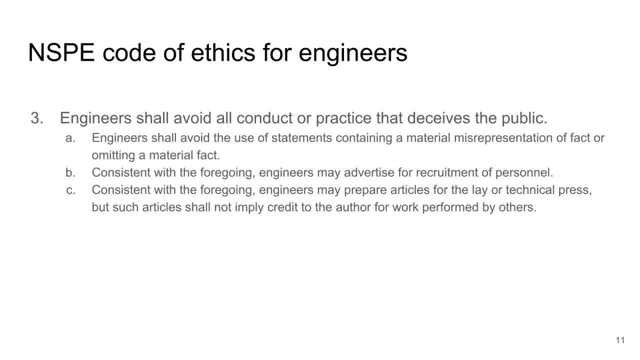 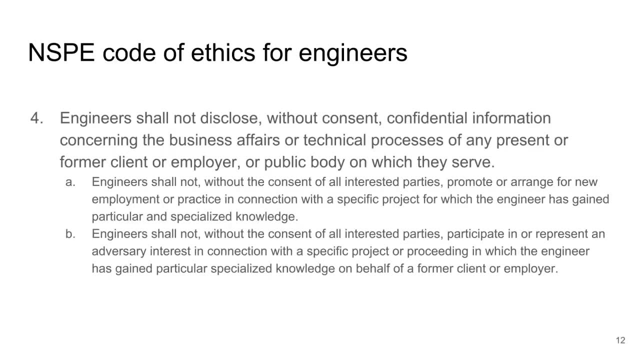 done, but also the ideas. if someone had an idea for how to do something and then you implemented it, you need to give credit for where the underlying ideas came from. point four: engineers shall not disclose, without consent, confidential information concerning the business of the company or the company of the company or the company of the company of the. 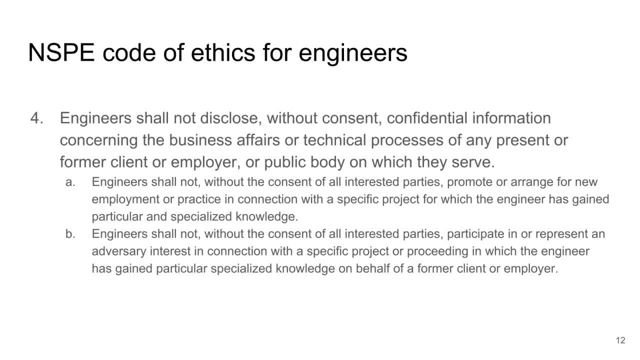 business affairs or technical processes of any present or former client or employer or public body on which they serve. so you're being told you need to keep confidence when you are on a panel and a panel makes a decision you can't then go talk to the press about. you know where. 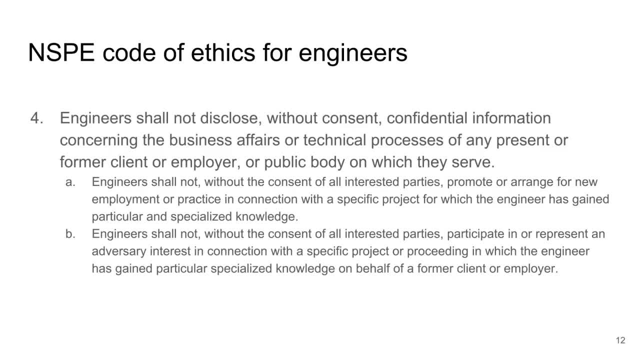 this decision came from. uh, let's go through a and b here. uh, a engineer shall not, without the consent of all interested parties, promote or exchange or arrange for new employment or practice in connection with a specific product for which the engineer has gained particular specialized knowledge. b- engineers shall not, without consent. 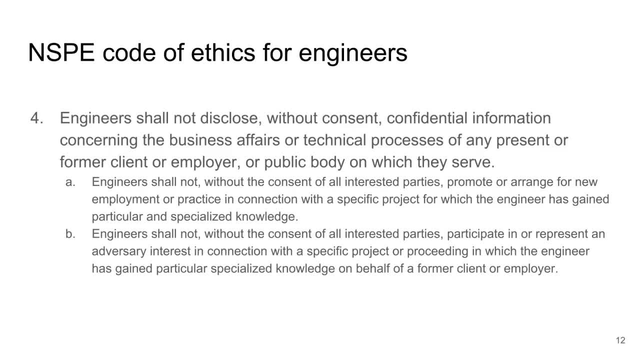 of all interested parties participate in or represent an adversary interest in connection with a specific project or proceeding in which the engineer has gained particular specialized knowledge on behalf of a former client or employer. so not only are you supposed to keep confident, but you're also supposed to avoid future conflicts of interest, whether it's you looking for work or 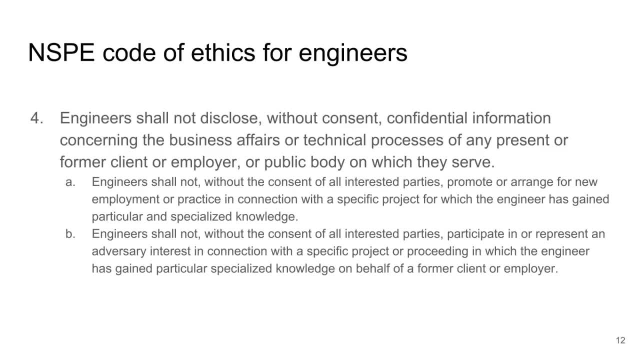 you know, for example, working on other boards or committees for the public, when an employer hires you to make a specific product, then you're forbidden from seeking employment. uh, based on fat specialization, right. so say, an employer or someone who's a someone else wants to hire you to deconstruct or to make a competing product, and you're forbidden. 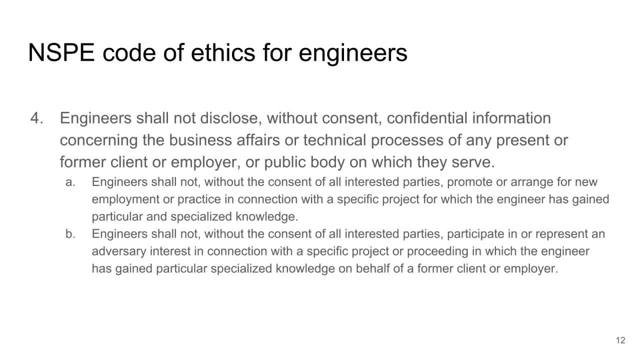 from that and, fortunately, most the time you also have a non-disclosure agreement you sign with your employer. but even if you don't sign a non-disclosure agreement, according to our code of ethics as engineers, you're not allowed to use what you've learned to. 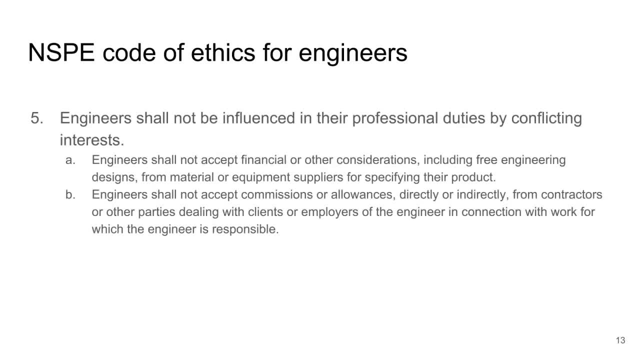 profit. point five: engineers shall not be influenced in their professional duties by conflicting interests. point a: engineers shall not accept financial or other consideration, including free engineering design, from materials or equipment suppliers for specifying their products. engineers shall not accept commission or allowances, directly or indirectly, from contractors or other parties. 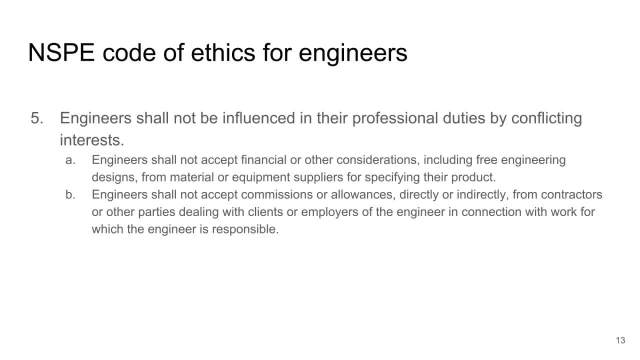 dealing with clients or employers of the engineer in connection with work for which the engineer is responsible. basically, here you're saying that engineers are not allowed to be influenced by their professional duties by conflicting interests. point five: engineers shall not be influenced in their professional duties by conflicting interests. point a: engineers shall not accept financial or other consideration, including free engineering design, from materials or equipment suppliers for specifying their products. engineers shall not accept commission or allowances directly or indirectly from contractors or other parties dealing with clients or employers of the engineer in connection with work for which the engineer is responsible. 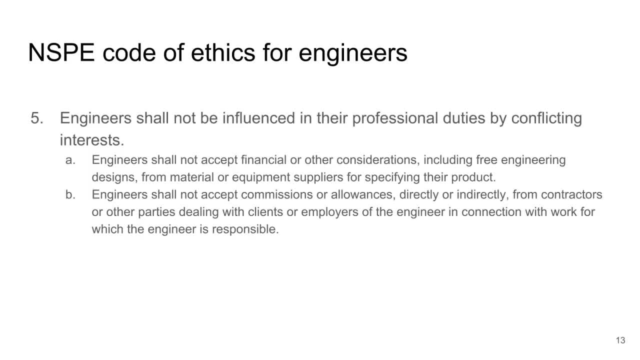 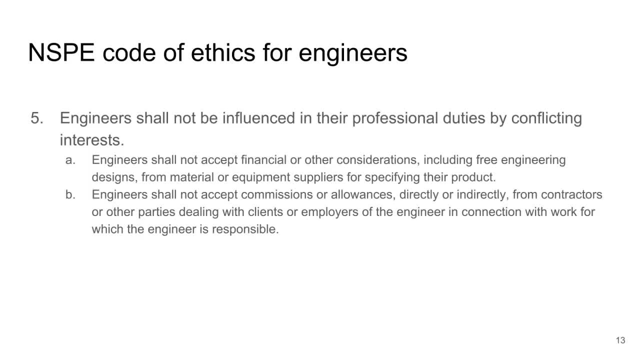 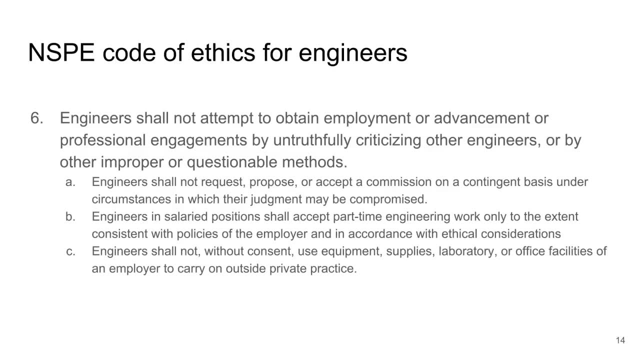 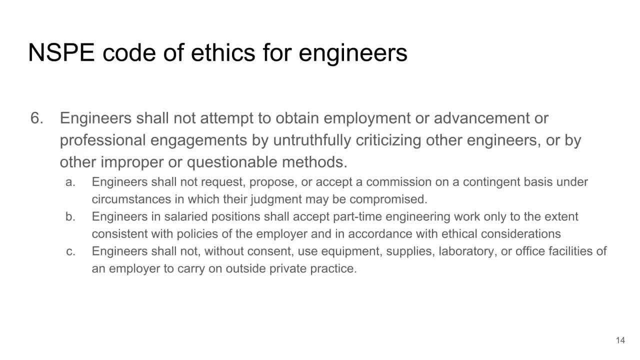 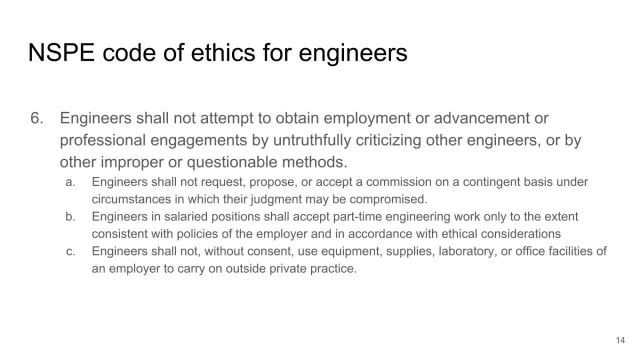 may be employed, but you will not take part-time employment on the side that compromises your work as an engineer. that, for example, uses your employer's equipment, that uses your employer's name or by any other form, violates your agreement with your employer, and most of the time, employers have. 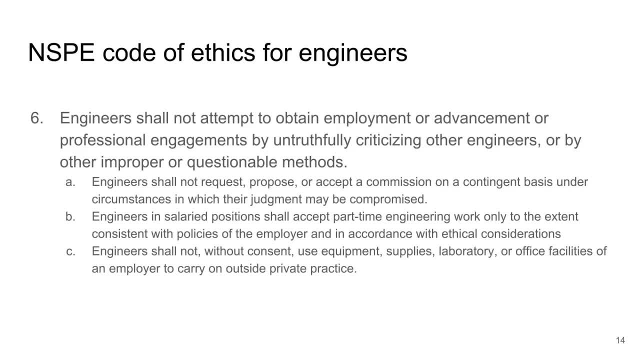 rules. so, for example- uh, you know, professors, we are given a certain number of hours per year that we are allowed to do contract work and we have to stay within those, and we're also told about intellectual properties that come from our work, and these are all in our contracts. 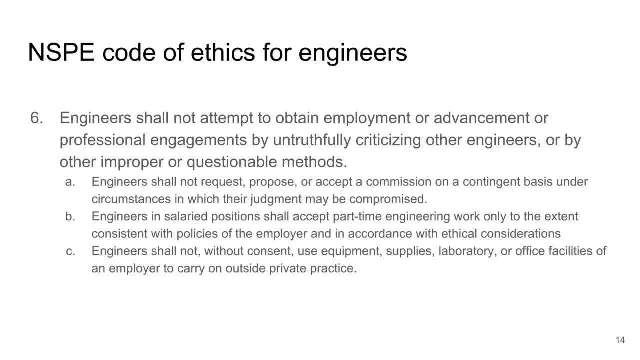 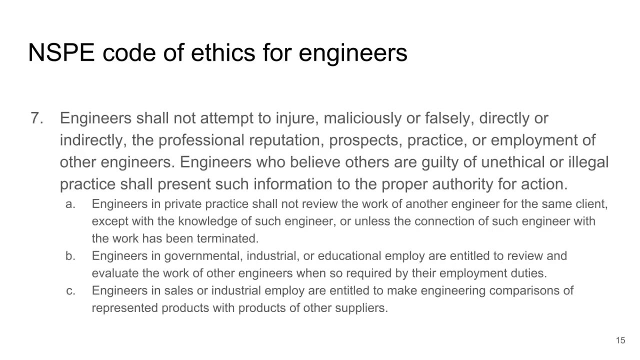 so it's something that if you're working for a firm, then, as an engineer, you need to be aware of what these rules are and to act accordingly. point seven: engineers shall not attempt to injure maliciously or falsely, directly or indirectly, the professional reputation, prospects, practice or employment of other engineers. engineers who 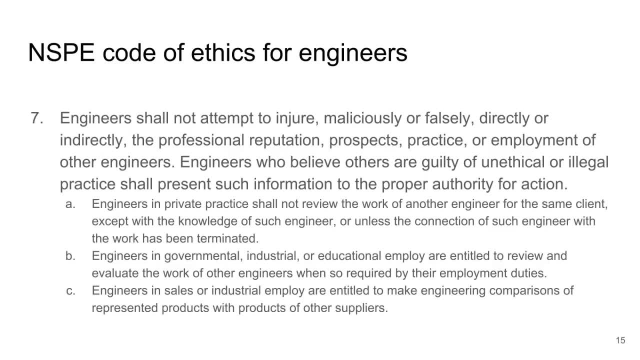 believe others are guilty of unethical or illegal practices, shall present such information to the proper authority for action. point a: engineers in private practice shall not review the work of another engineer for the same client except with the knowledge of such engineer or unless the connection of such engineer with the 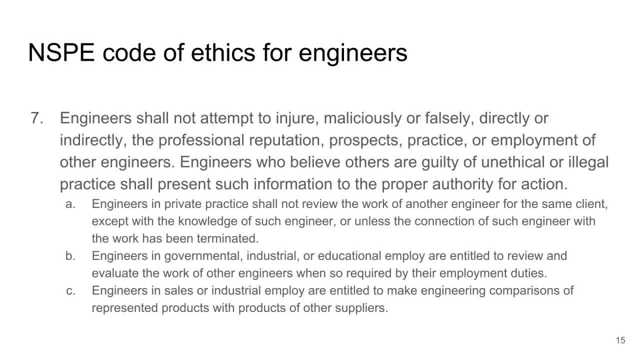 work has been determined. engineers in governmental, industrial or educational employee are entitled to review and evaluate the work of other engineers when so required by their employment duties. engineers in sales or industrial employer entitled to make engineering comparisons representing products with products of other suppliers. so, basically, you're not allowed to slander or libel. 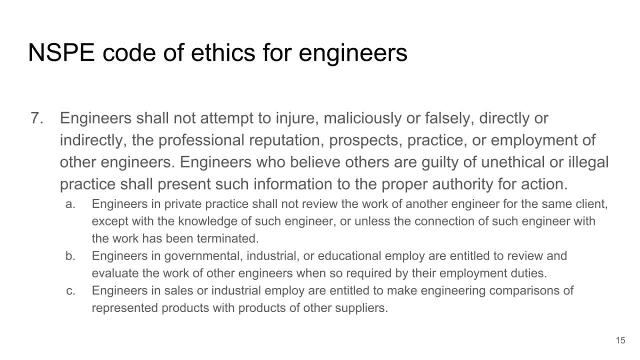 other engineers or other engineering products. so, for example, you're working for a company and you know the guy down the way. you think that he made some mistakes. well, you can't go back and double check his work unless your employer requests you to do that or unless, uh, he or she knows that. 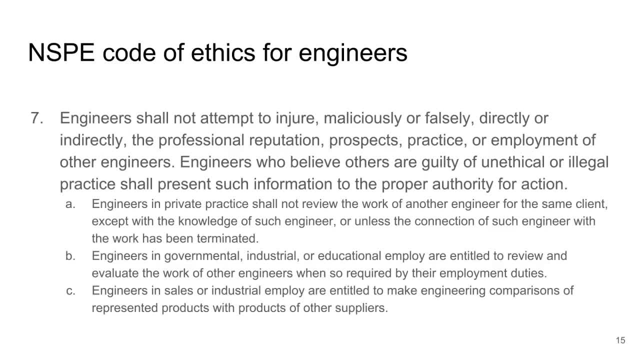 you are double checking their work right, and so you know. you're not allowed to review other engineers. for the same reason, you are not allowed to review other engineers. for the same reason, you are not allowed to review other engineers. and this is about. you know pretty much how you interact with other engineers, so you're not. 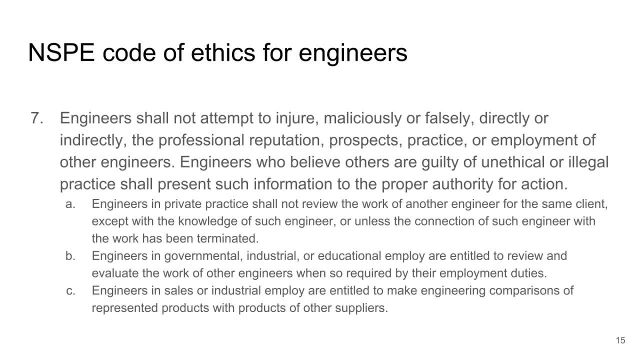 undercutting them in the workplace. you know you don't show up to a meeting and say: well, i know you know bob or mary presented this, but my results are different and my results are better. you know, even though they may be better, uh, it's still not. 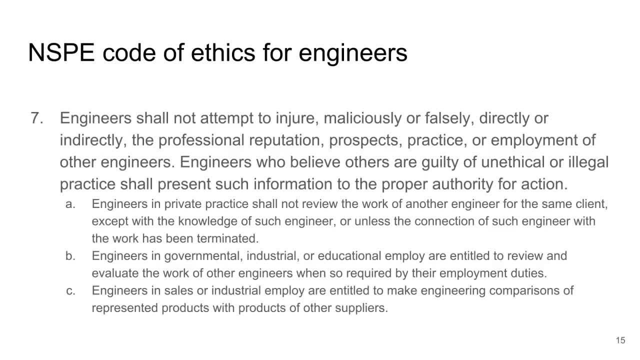 the same way, because you're not allowed to compare your competitors to your company. you can't compare your company to your engineer's work if your employer requires you to do so or if the person is no longer working for the company, and in the same way, you're allowed to. 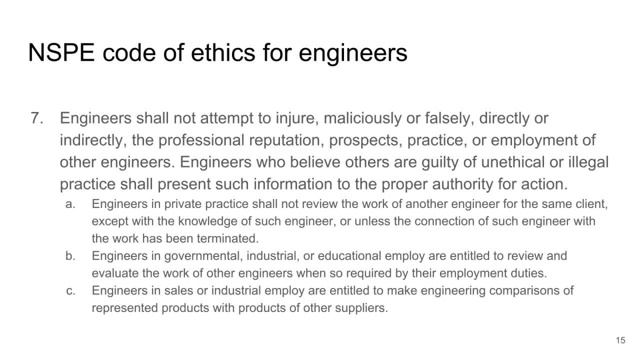 compare products from, say, your company and your competitors company. but there has to be a truthful comparison and this is both by what you say and by what you don't say. so you know, just because you don't say, that your competitor's product you know has some attribute which is better than yours. 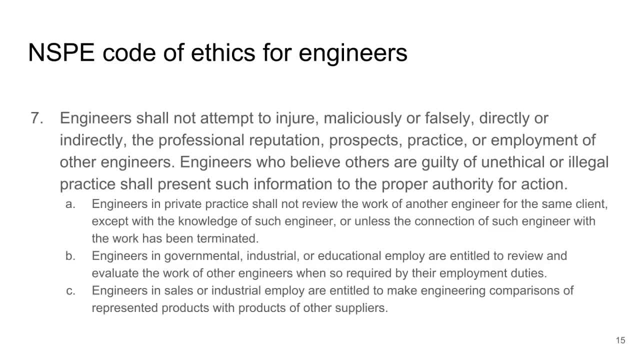 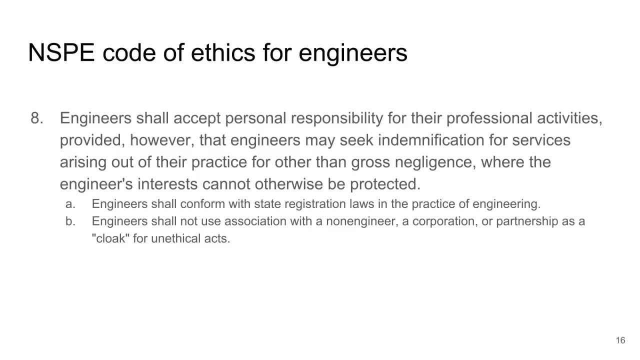 that doesn't make it right. you have to point out the advantages and disadvantages in as honest a fashion as you can point. eight, engineers shall accept personal responsibility for their professional activities, provided, however, that engineers may seek indemnification for services arising out of their practice for other than gross negligence, where the engineer's interest cannot otherwise be. 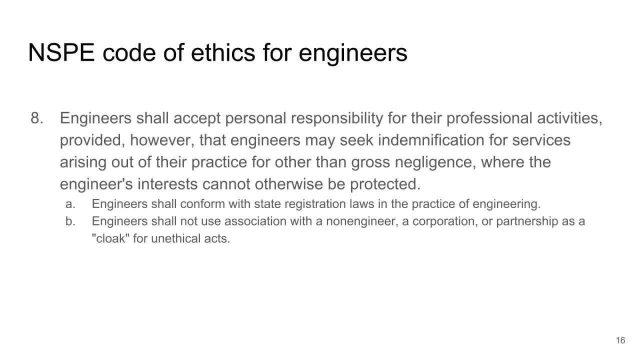 protected- point a: engineers shall conform with state regulation, regulation laws in the practice of engineering. point b: engineers shall not use association with non-engineers, a corporation or partnership as a cloak for unethical acts. so what this is about is basically saying that your actions are your own and you have a responsibility. 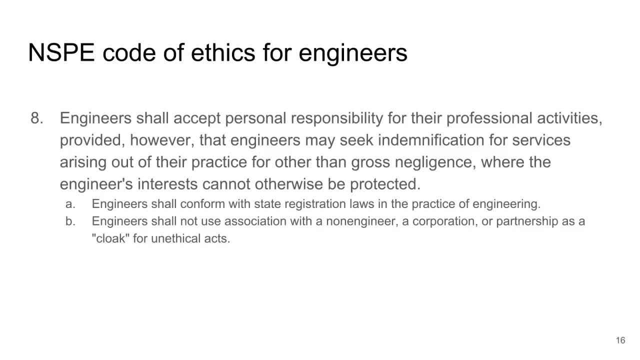 for your actions and you have a responsibility for those. uh, point b says that you can't hide behind a company. say: well, you know, i said that you know. this pharmaceutical drug, you know, can sometimes cause heart disease and it's up to my employer and the lawyers in my company to make. 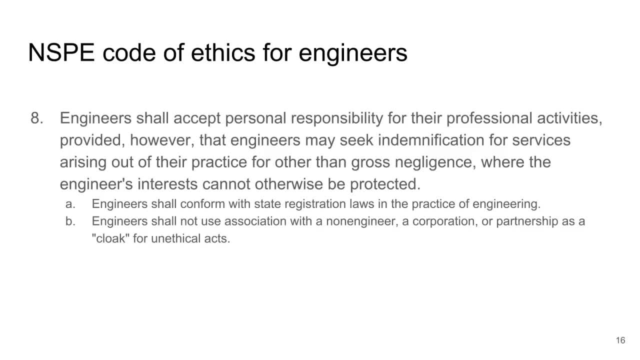 the statement. you know if you have that data, you're not allowed to hide behind the lawyers from your company to cloak you from unethical actions. you're still behaving unethically and you're not required to. you know work with state regulations in terms of how you practice. 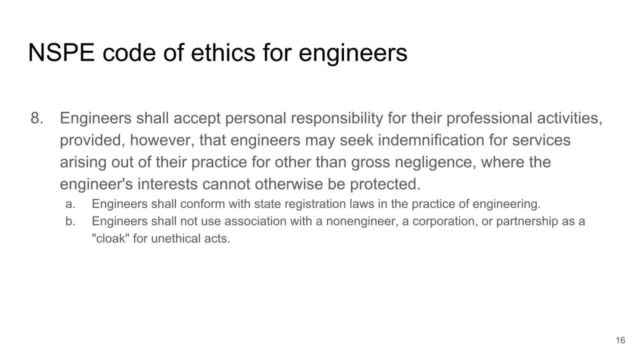 engineering, whether it's licensing or testing. now here we talk about indemnification for services, uh, and it's also telling you that your behavior is shielded somewhat, uh, from a litigation. so, for example, as long as you're behaving in an ethical and as long as you don't have gross negligence, then any lawsuits arising from your services, 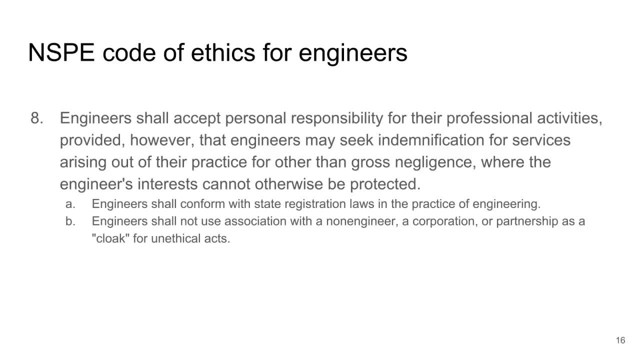 you are protected from or you should be protected from. you know so. for example, say, you are working on the braking system of the automobile. you've, you know, tested it according to engineering standards. you know that they're safe, you certify them. if something happens- and this is might be. 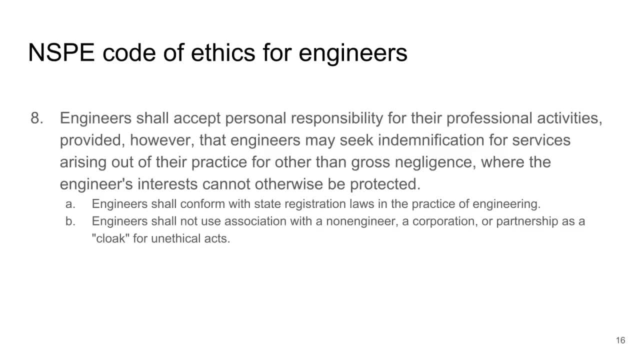 for example, during the processing or maybe a material supply or something, and there is a lawsuit due to the brakes failing. you should be protected as long as you've behaved ethically, and that ethical behavior also means that you can't, you know, mask failures by passing it to the lawyers. you need to be upfront about that. 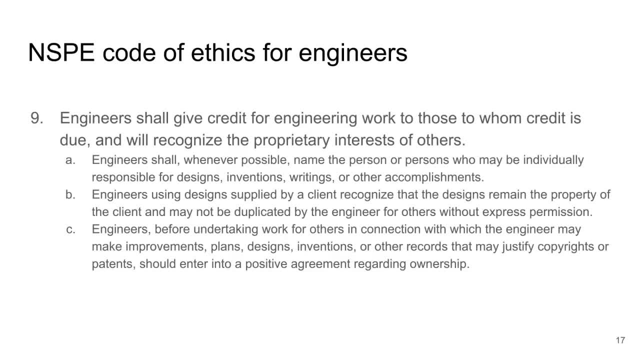 point nine: engineers shall give due credit for engineering work to those whom credit is due and will recognize the proprietary interests of others. so this is really again a statement against plagiarism. it says, point a: engineers shall, whenever possible, name the person or persons who may be individually responsible for designs. 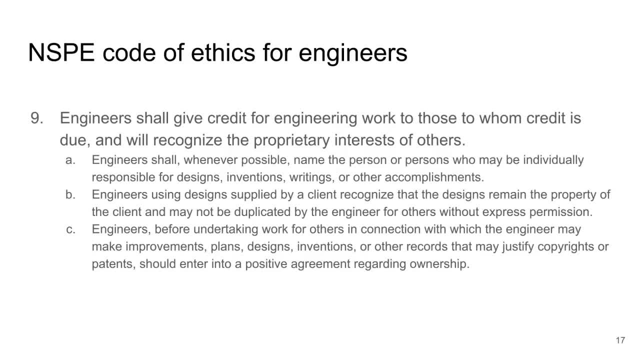 inventions, writing or other accomplishments. you know you don't necessarily know the origin of certain designs if you're working within a company, but if you do, even if the person is no longer working with a company, you need to to recognize what they've done. point b: engineers using designs supplied by a client recognize that the designs remain the. 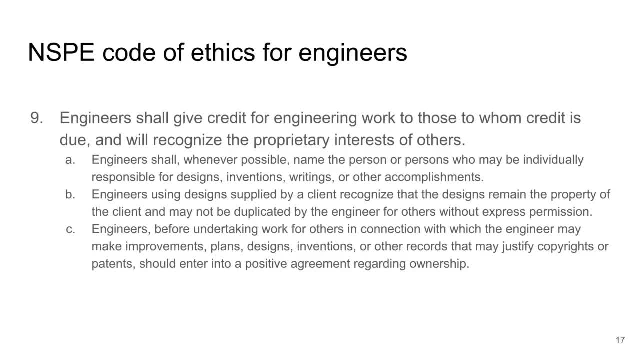 property of the client may not be duplicated by the engineer for others without express permission. so this is about intellectual property and if you're using a company's ip, it remains their ip, a unique place to work. we would think about it having like lines that relate to the. 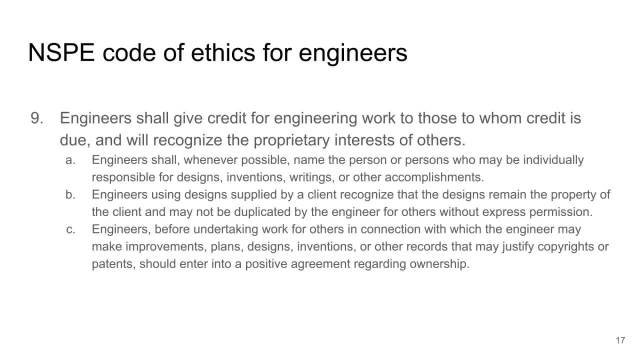 different highway bypass lightspopcars. that jetzt really deals with the distribution of property and therefore fact-checking efforts from the industry. point c: engineers. before undertaking work for others in connection with which the engineer may make further improvements, plans, designs, innovations or other record that may justify copyright, a patent should enter a positive agreement regarding ownership. so this is basically saying that when you start working, you need to have the intellectual property ownership established and what you can and can't do. so, oh, that you can't do, so you need to coexist and be able to have what you're saying sorted out. bueno, 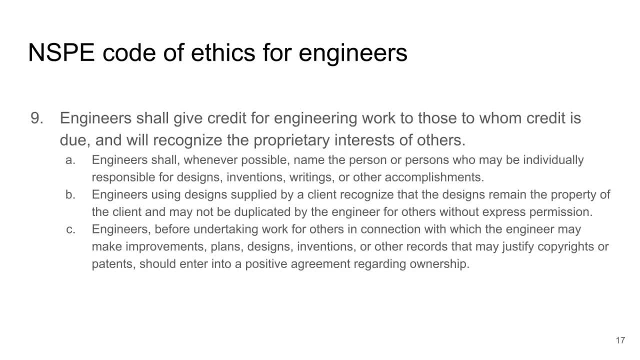 So, for example- again, professors, we work for the state and in our contracts we have an agreement about intellectual property. So if we design an invention and patent this, there are rules about how we can use it, if we can license it, who we can license it to and how profit goes with that. 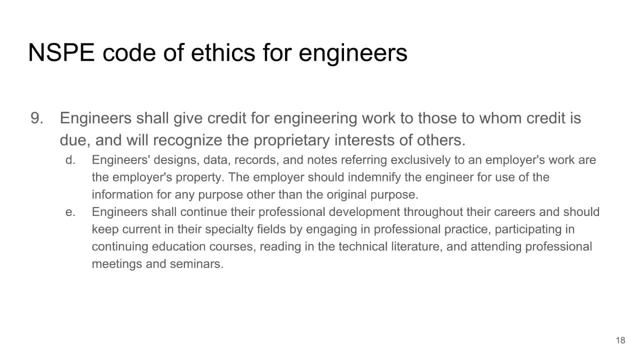 Point D: engineers design data records and notes referring exclusively to an employer's work or the employer's property. The employer should indemnify the engineer for use of the information for any purpose other than the original purpose. So what you do for a company stays with that employer. 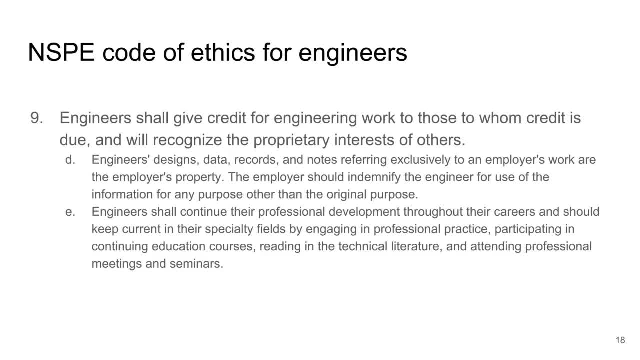 And this last part about indemnification. this is saying that, for example, your employer hires you to design skateboard wheels And you do this, you leave the employer or you move to another project and the employer takes that design and they say: 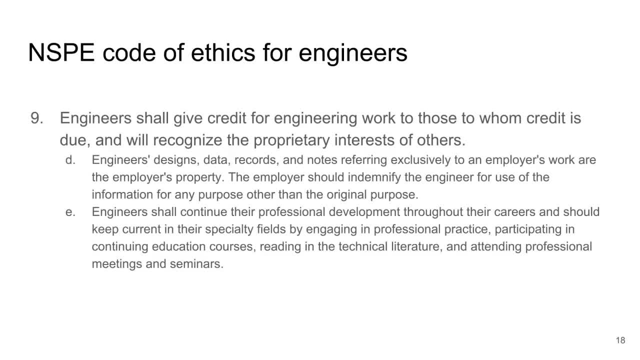 oh, now we're going to use this for equipment for moving heavy machinery And you say, well, that may or may not work, but you should be protected from their use of the design that you left with them And you're not ethically responsible for this. 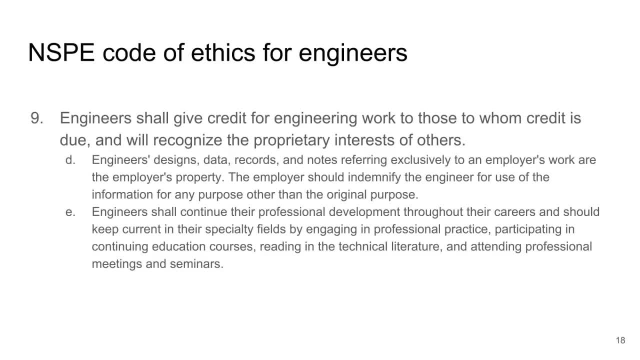 This is something that is outside of your control. E engineers shall continue their professional development throughout their careers and should keep current in their specialty field by engaging in professional practice, participating in continuing education courses, reading in the technical literature and attending professional meetings and seminars. 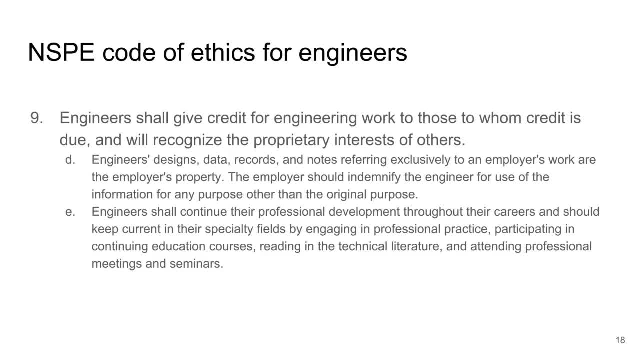 So you have a responsibility for lifelong learning, right? You're specialized. You're specialized in, again, designing wheels or skateboards. Well, that's going to change over time. And then your job as an engineer, your duty as an engineer, is to keep up in the current design. 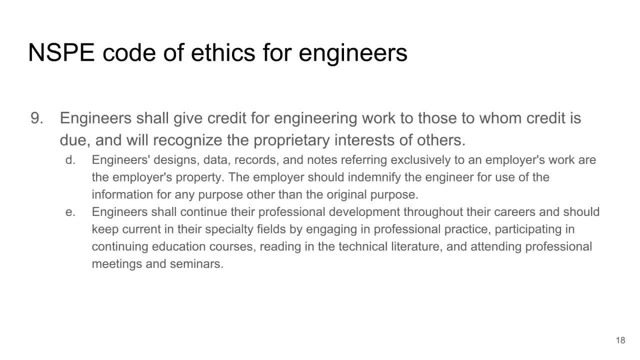 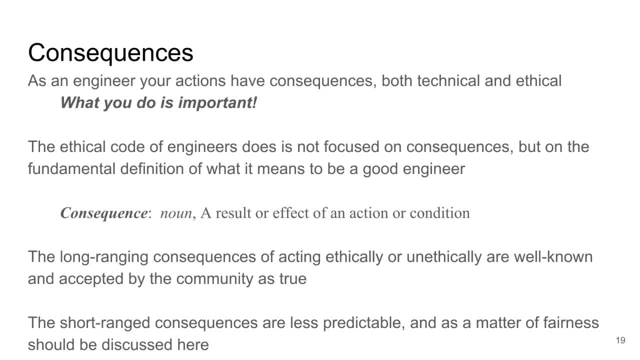 So these nine points and the canon, these are from the NSPE Code of Ethics. Now, what you do as an engineer has consequences. There's consequences for what you do, both technically and ethically, And this is because what you do is important. 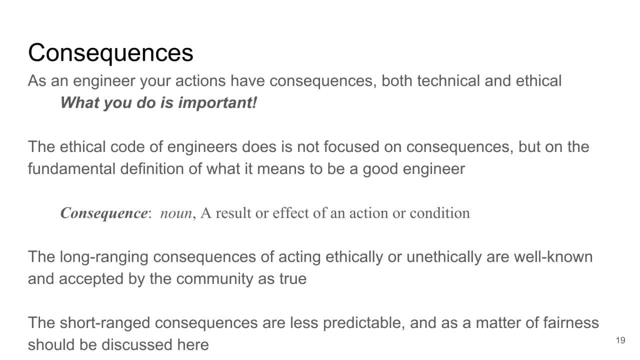 The preemblem to the Code of Ethics states: you know, what you do as an engineer is important And that's why there's consequences for this. Now, as engineers, we don't focus on the consequences And we focus on being good engineers. 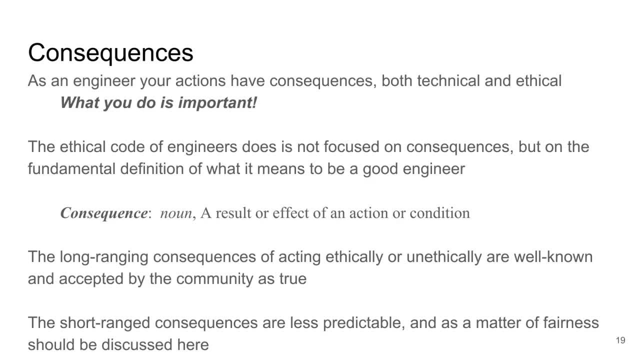 You know the consequences. They're the result. They're the result of an action or condition. So in my opinion, when we teach engineering students that you know we behave ethically because you know it's important for the safety of the public, that's not exactly true. 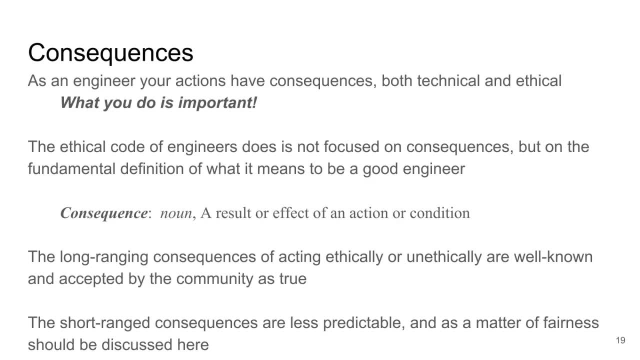 We behave the way we do because it's what it is to be an engineer And we have a long-range perspective. This is what our Code of Ethics tells us about. We're not focused on the consequences. Now, these long-range consequences, they're well-known, right. 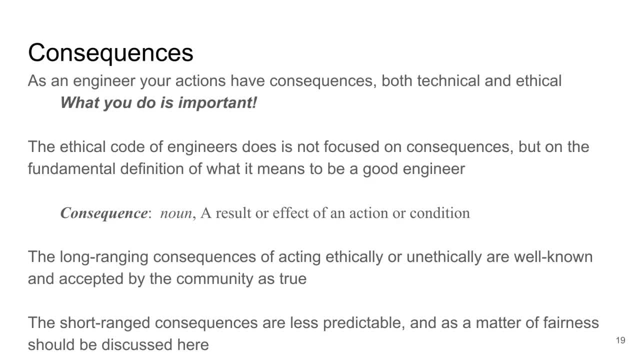 If you behave as an engineer in an honest fashion, technically and ethically fashion, in terms of how you design and how you look at the future, how you look at environmental considerations, how you look at the overall health and welfare of the people, you're not focused on the consequences. 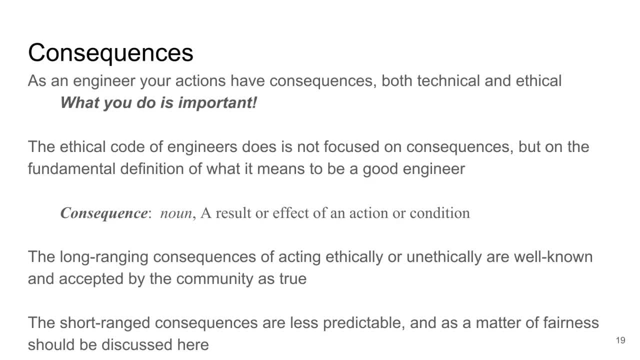 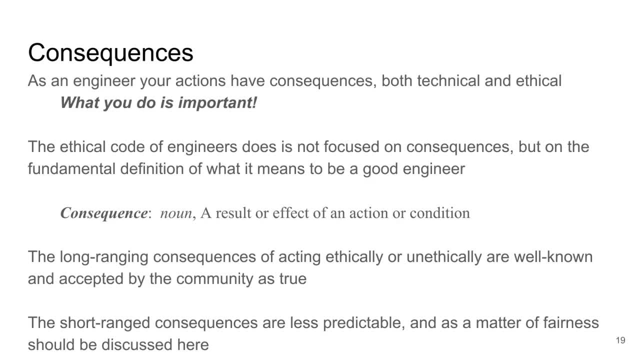 So I want to talk about those here, just as a matter of fairness. But you know, you should know, that the consequences of your actions from an ethical perspective are a little bit unpredictable. You know so the consequences of you doing the right thing. 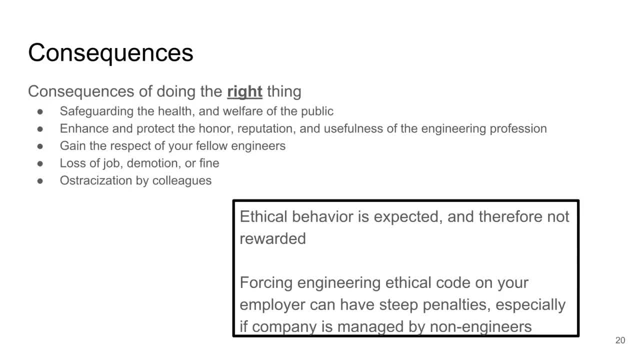 and behaving like a good engineer is that, of course, you're going to safeguard the health and welfare of the public And you're going to enhance and protect the honor, reputation and usefulness of the engineering profession We don't have. you know there's jokes about. 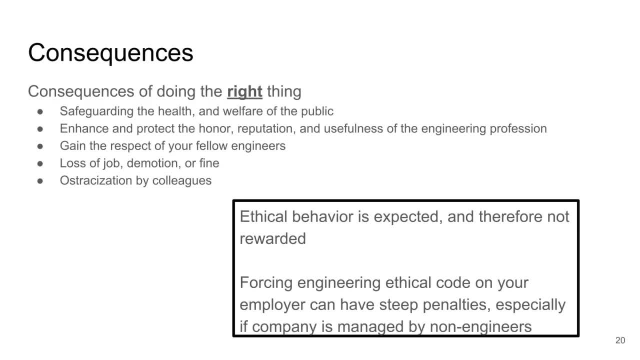 you know lawyers, and the lawyers are always kind of the butt of the joke. We don't have that about engineers. Engineers are, in general, respected by the public because good engineers- and there have been, you know, generations and generations of these- 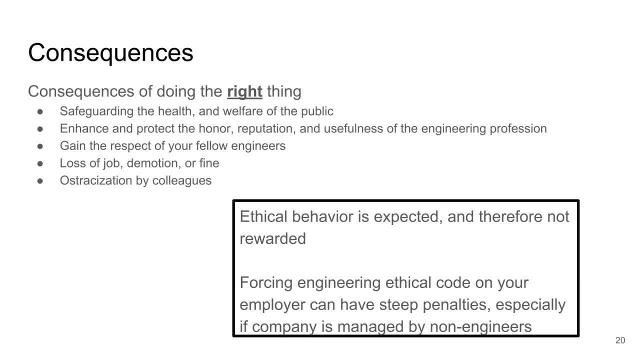 good engineers. they do right by the public. If you do the right thing, you're going to gain the respect of your fellow engineers. Now, if you do right, other things may happen. For example, doing right may mean that you lose your job. You may be demoted by your employer. You may be fine. 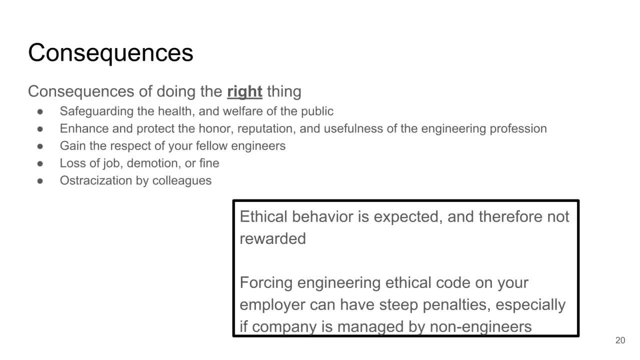 by your employer. You also may be ostracized by your colleagues. What do I mean? I mean that if you do what's right as an engineer, particularly if you are working for a company that's managed by non-engineers, your actions may be viewed as damaging And people may think, oh my gosh, I don't want to work. 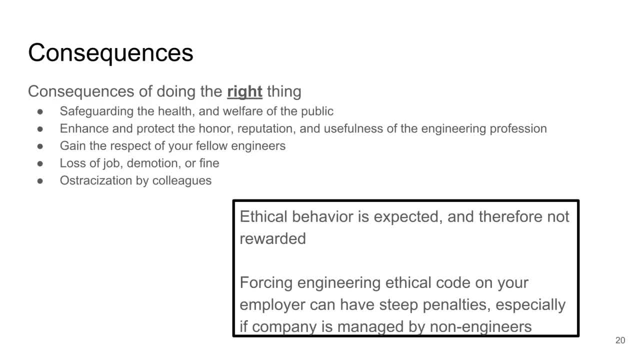 with this person. There's such a pain in the neck. Every time that I propose a solution, they say no, we can't do that because there's some you know ASTM standard that violates, So I don't want to work with them. 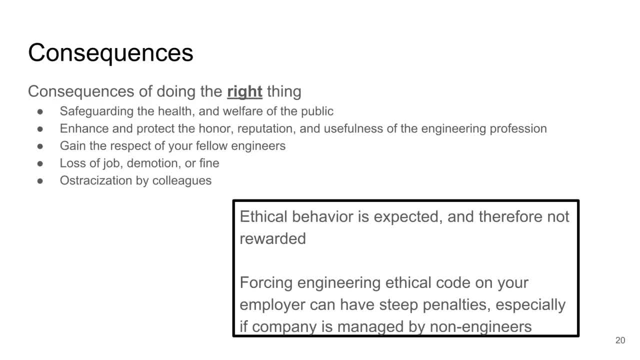 Well tough. That's a consequence of doing the right thing. It's a consequence of looking out for the health and welfare of the public. But these are the short-term consequences. The long-term consequences of doing the right thing is definitely a win. It's a win for you. 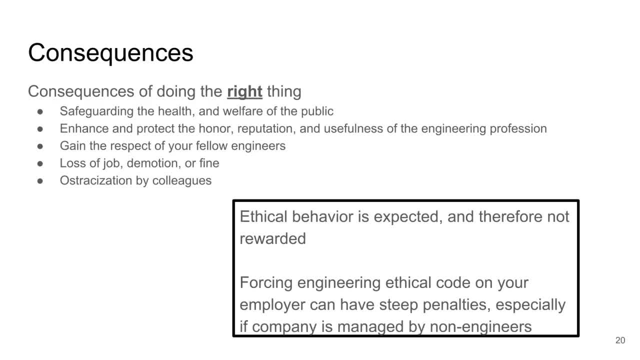 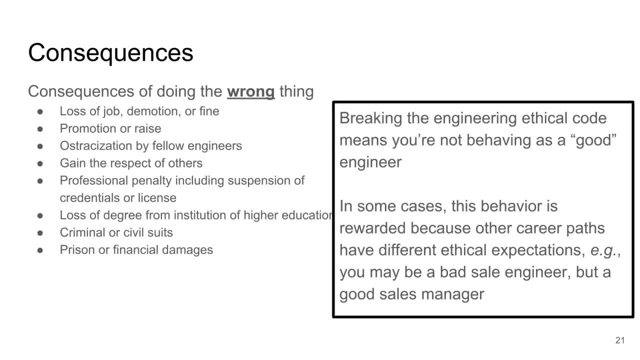 and it's a win for you know humanity on the whole. But short-term you may have difficulties. Now there's consequences for doing the wrong thing. If you do the wrong thing, you might lose your job, You might be demoted, You might be fined. 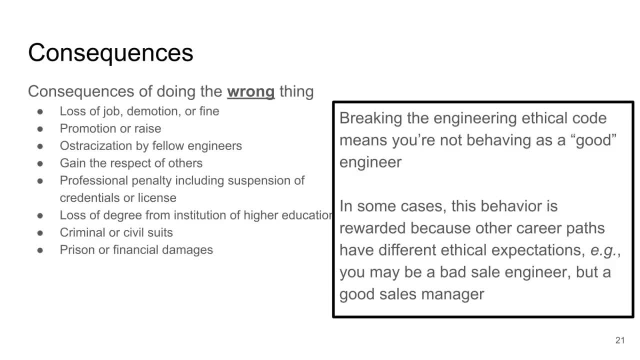 You also might get a raise, You might get a promotion. Your fellow engineers may ostracize you for doing the wrong thing. Say, well, yeah, I saw him and he or she- they you know- made shortcuts and they didn't follow the standards. And your fellow 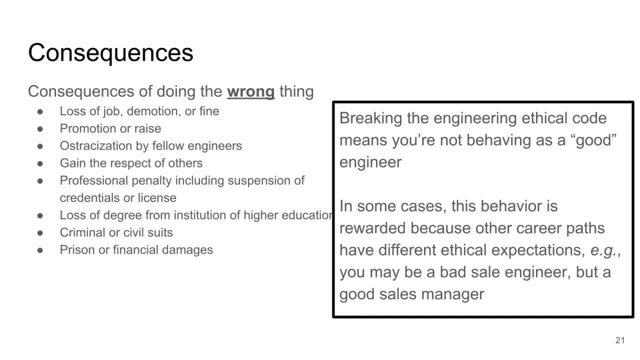 engineers may not want to work with you, So if you do the wrong thing you might lose your job. to work with you, they may report you to the uh nspe uh. but you also may gain the respect of others. you know, you know he or she came up with a really great idea for, you know, circumventing. 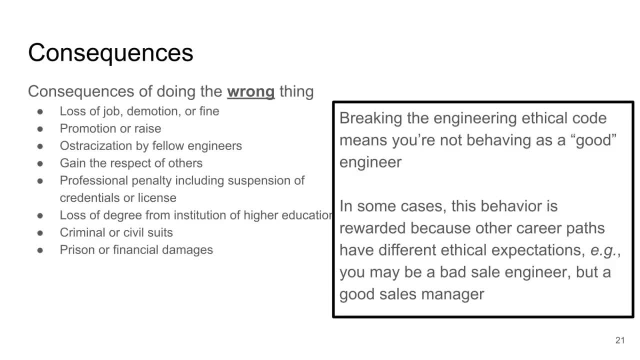 this market problem we had. you know these are non-engineers, but these non-engineers may have you covered in their engineering job um yourself and they may shaped your business life or you have a job for yourself that you can support, but you don't necessarily know. 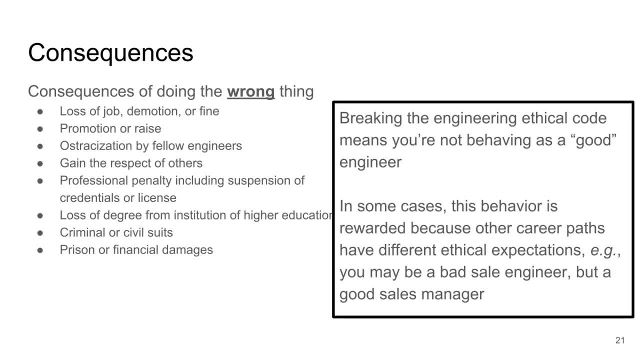 whether the die may help you. you may receive professional penalties. you may be suspended. your license may be suspended. your credentials may be revoked. there have been cases where engineers have lost their degrees from. You behave unethically and you produce a product that is dangerous, that endangers people's lives. 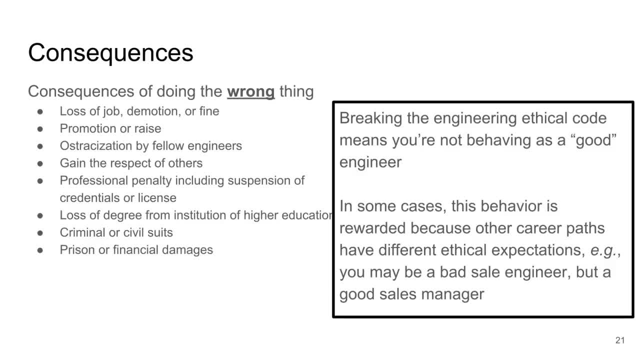 This could lead you to wrongful death suits. Things go very badly. You could be liable for a wrongful death. You could even wind up in prison for manslaughter for your behavior. So in general, here being a good engineer and doing the right thing, the short-term consequences are up and down. 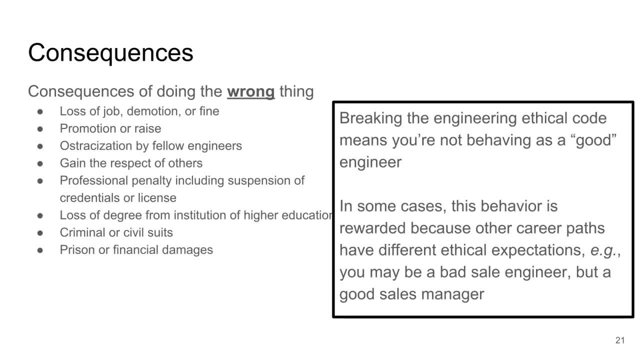 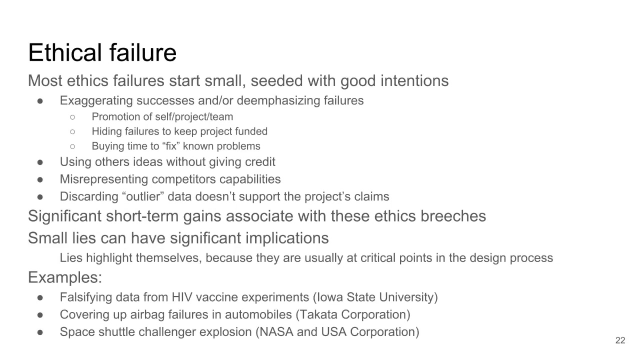 The short-term consequences of doing the wrong thing, also positive and negative, But we know that in the long term, being a good engineer means behaving ethically, And this is where we're going to have the greatest gain for society. So thinking about how engineers fail ethically. 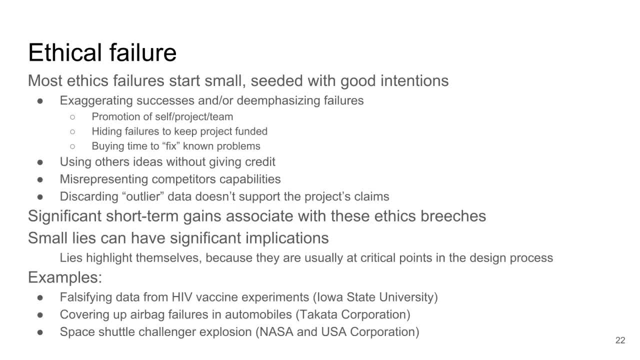 Most engineers. where they fail, they don't plan a large-scale ethical breach. No one does that, Almost no one. I'm sure there's some sociopath that might, but most of us no, we don't. It starts out with something small. 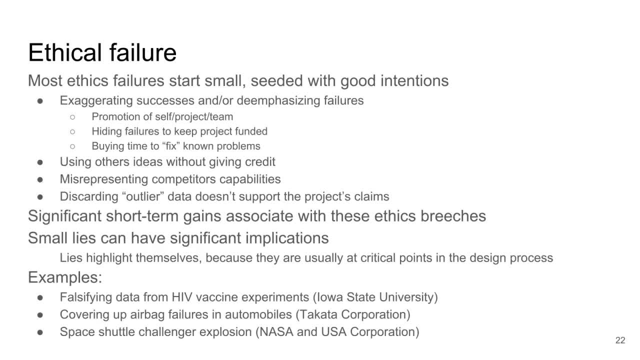 You may exaggerate your successes or de-emphasize your failures, And in doing so you'll get a promotion of your project and your team. It might be that you have a project that's working except for one little part and you hide that part. 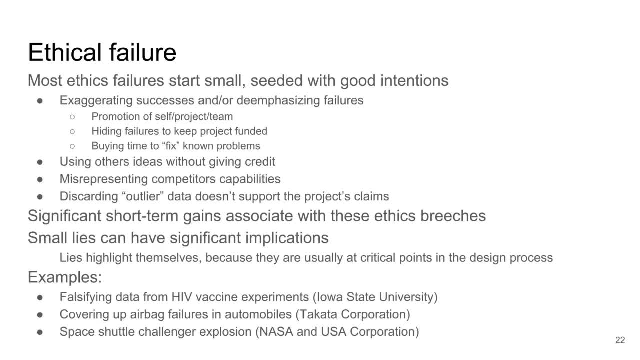 So this is an ethical failure by not being honest, by not telling all of the material failures, And you do that because you know that you're not going to be able to do it. You know that if that failure comes up, they're going to defund the project. 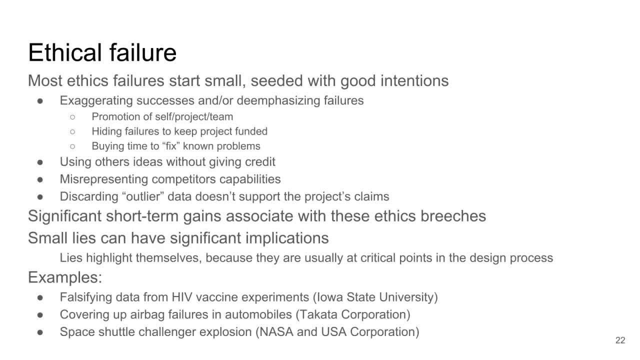 People are going to lose their jobs, The company may lose contracts And you're going to hide this because you know that with enough time you'll get a fix. You'll know how to solve it. That's a form of ethical failure. 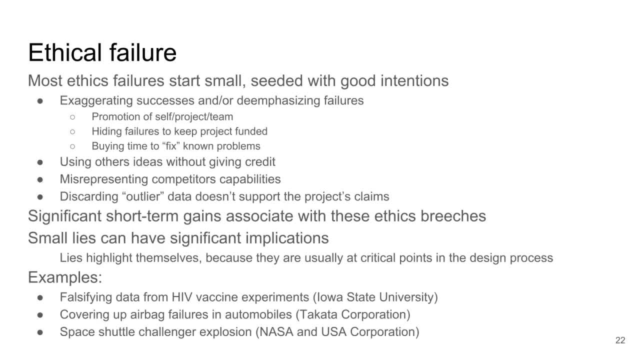 Another form is plagiarism: Using other people's ideas without getting credit. You say, oh, I borrowed the idea. Well, no, you didn't, You stole the idea. But that's a form. That's a form of ethical failure. 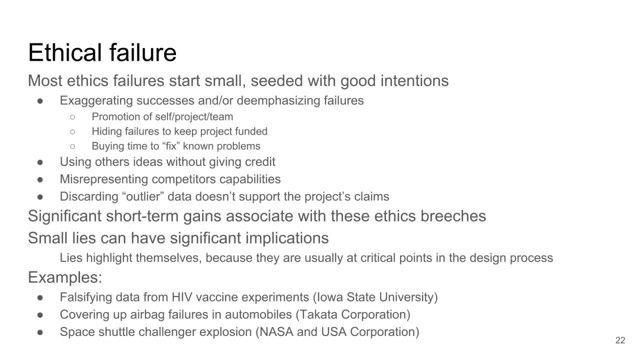 And, it happens, Misrepresenting competitors' capabilities. Again, this is about competition And as time has gone, the competition has gotten steeper and steeper. We're not just competing nationally, We're competing internationally, And the bottom line of products is a big deal. 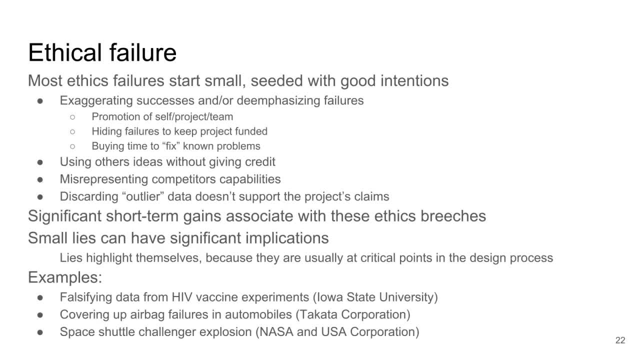 So there's a real temptation to misrepresent Your competitors in order to gain an advantage. Another example is discarding outlier data that doesn't support your product's claims Or project's claims, And there you know, there's reasons that there really can be real outliers. 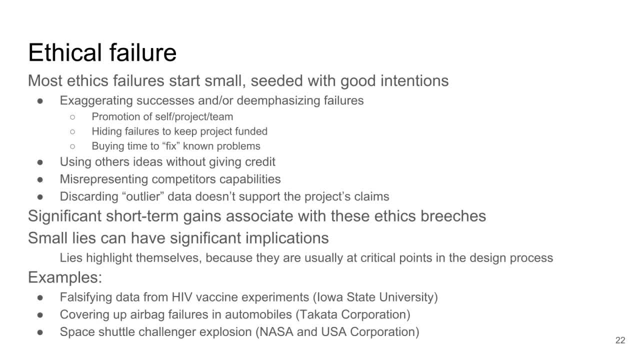 But you have to have evidence that those are real outliers. You can't just say: well, you know, this looks good, except for these three data points, Let's get rid of those. So these are all small failures, But these 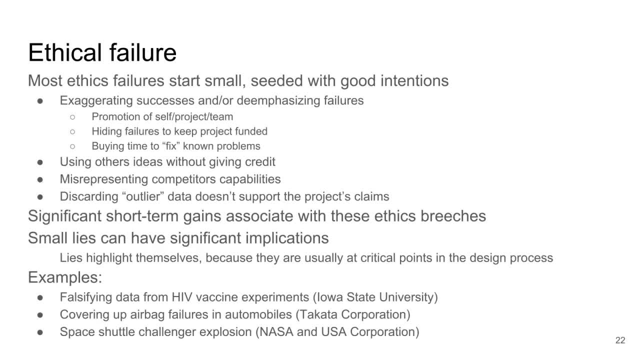 Small failures, So these small ethical breaches. they will give you short-term gains, But these lies, they always catch you And the reason that these type of lies you get caught in is because no one lies about something inconsequential, Right. 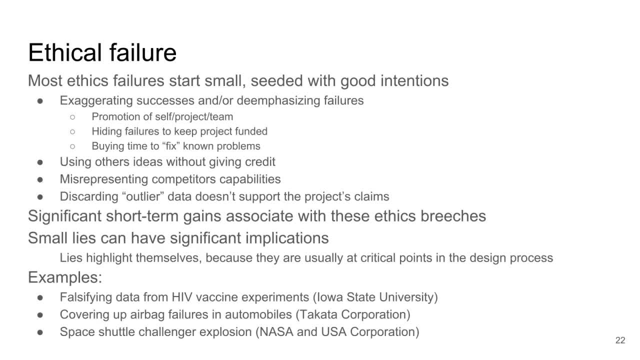 You make a lie about you know this product works great, except that you know it causes your hair to fall out Or whatever. Right That lie, it's going to highlight itself Because it's something critical, So you need to be careful of that. 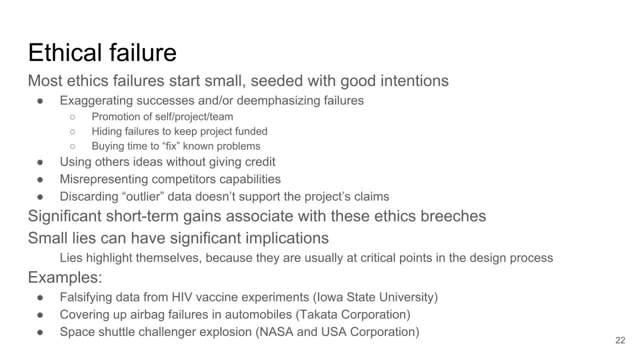 Because You are going to get caught, And I have some examples here. There's one example: Iowa State University. there was a professor in I can't remember which department, But he falsified data from HIV vaccine experiments on rabbits And he did this because if he didn't falsify that, he would have lost funding. 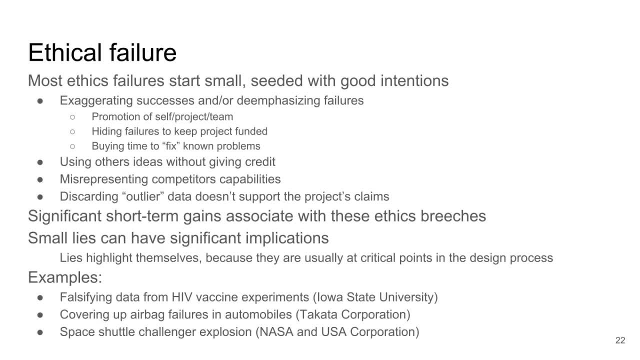 And that loss of funding represented, you know, graduate students, postdocs. It represented, you know, pretty much his life, His livelihood at the university. Now, falsifying that data meant that literally millions of dollars went into vaccine trials that were doomed to be failures from the beginning. 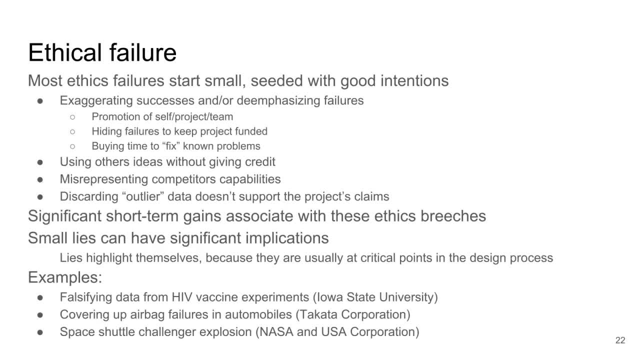 And those are millions of dollars that could have gone into other ideas. But this fraud, you know, protected himself And you know, I don't know if this person was going for tenure at the time, But it was a significant failure. 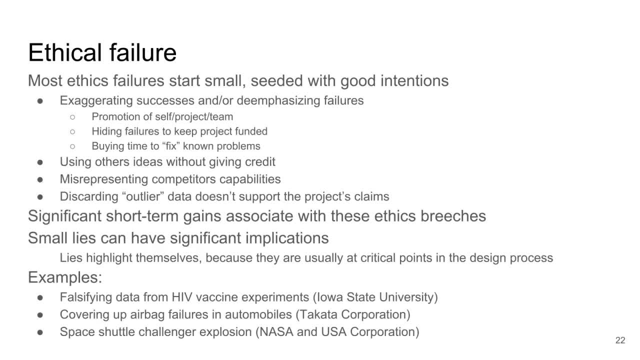 Another example was covering up the airbag failures in automobiles. This was the Takata Corporation And they had airbags that when they went off, they would spew hot metal on the passengers, And it was covered up for years Both by the company that was making these and the cars that were putting them in there. 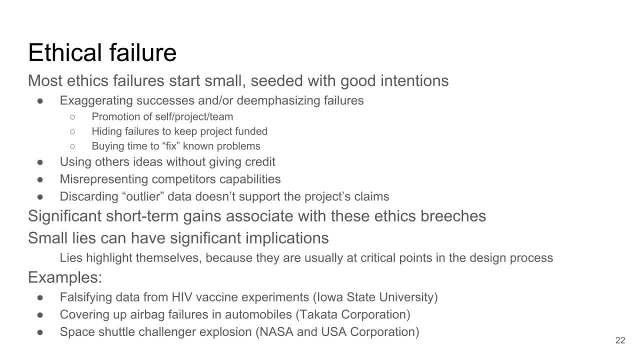 You know there was loss of life in this And the engineers involved in it. You know they may say, Well, you know I reported this to my supervisor, but that's not enough. They failed because they let public health and safety lapse, hiding behind the management structure and the lawyers in their company. 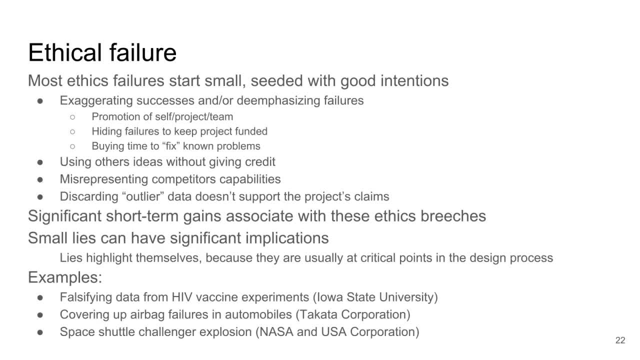 And the third example was the Space Shuttle Challenger explosion Right, And this was NASA and the USA Corporation, which is the United Space Alliance. there They were responsible for Preparing launch vehicles And basically they had a part that they knew underwent a. 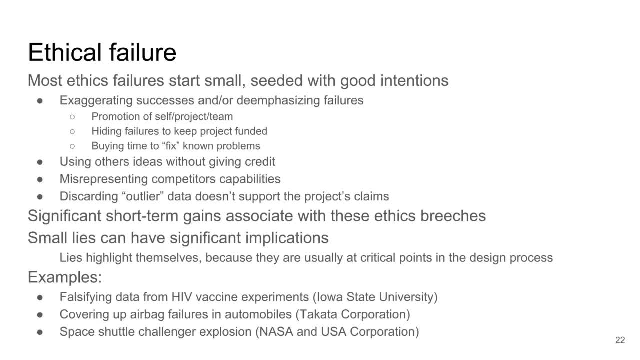 Ductile to brittle transition below a certain temperature And the O-rings in these seals. And You know the question came up. you know, do we launch the space shuttle? And this was a high profile launch because we were putting a civilian up in a space- 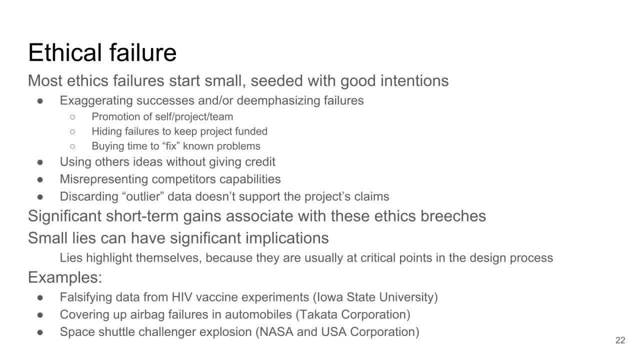 And they said, oh sure, go for it. I mean somewhere. I'm sure There were engineers. No, these parts aren't, aren't rated. And in fact those engineers- they were identified later that they had taken their concerns to management, but it stopped at that point. 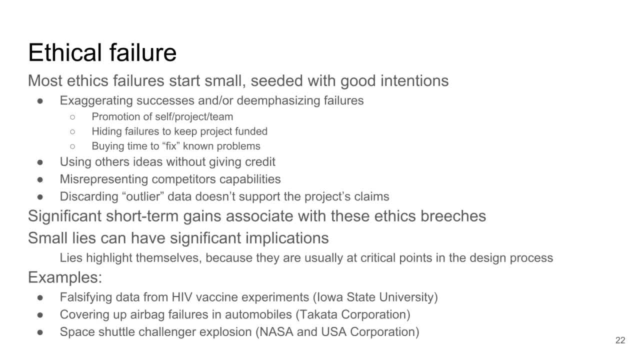 The people above them overwrote their their concerns, And we go back to the NSP rules of ethics. One: if your concerns about the health and safety of the public are overridden, then you're responsible. You're responsible for alerting the proper authorities, and the engineers did not do so. 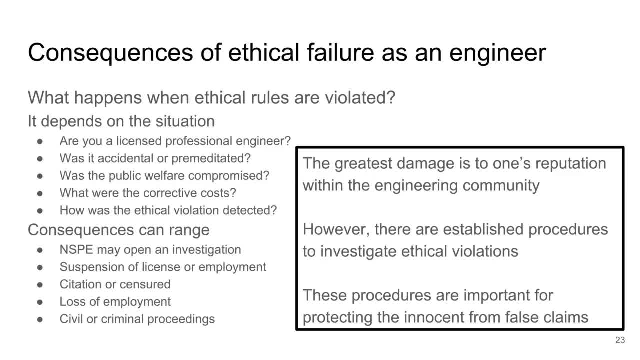 What happens if you violate ethics? Well, you lose reputation, and that that's. that's a big thing. But we have we have a set of processes by which Violations are are investigated, and it's important that you follow these procedures. A lot of these have to do with, you know, being a licensed professional engineer, but it is also within other professional societies that look at what you've done. 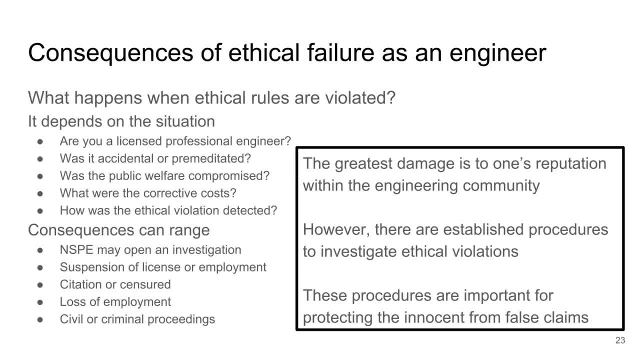 And it's important that we follow these procedures because we don't want to come to a situation where, you know, rumors are what govern penalty, And so when we say that we want to have a fair investigation of people's behavior from peers within their community, 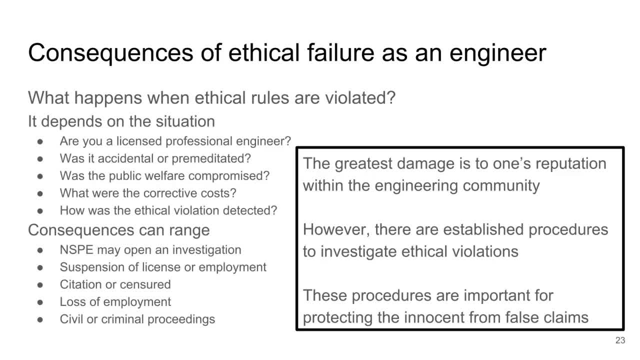 So announcing, for example to the that you believe there's been an ethical violation of a colleague or an employer, They can open an investigation And if you're a licensed P, You will be listed in the court as a licensed professional engineer. 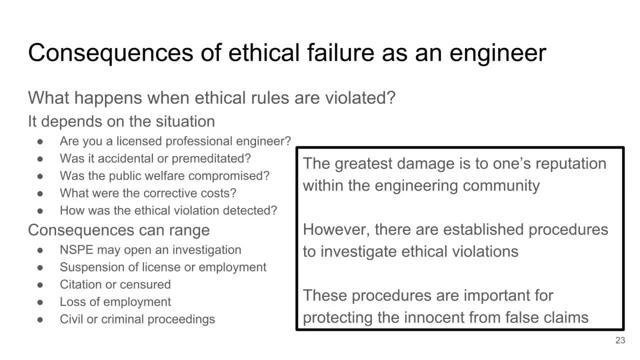 be listed as being under investigation. if you are being investigated and upon the conclusion you may be cleared, you may be suspended. your employer, depending on on the rules of your state, may have to suspend you. you may receive a censure from your company or from the professional. 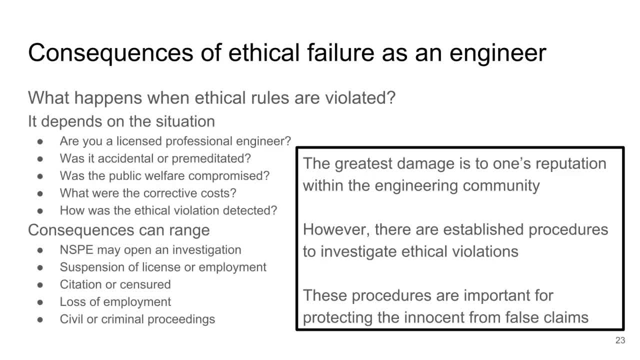 societies, you may lose your job and you also may be subject to, uh, similar criminal proceedings for for what, um, you've done. but this is something that the good news here is that we do have this, these engineering professional societies that will look at what's happened in a fair and judicious fashion. so 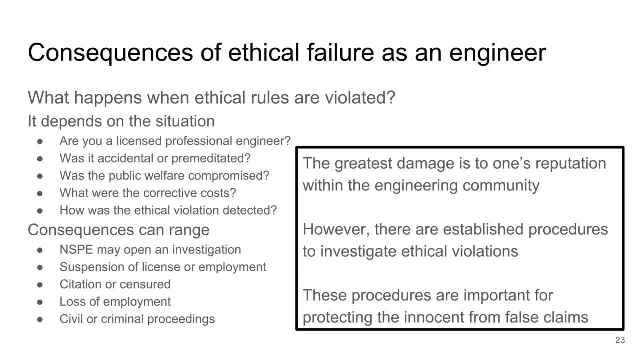 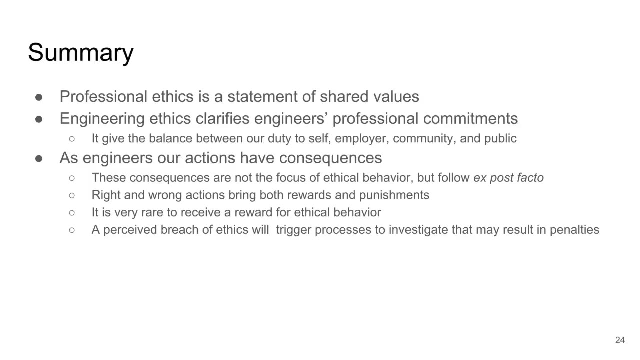 that's uh good news. if there is anything in the ethical failures- and a lot of times the failures themselves are- are considered within the context of: you know, was the public welfare compromised? what were the costs? uh, how did the ethical violation come about? so, in summary of of this discussion of engineering ethics, 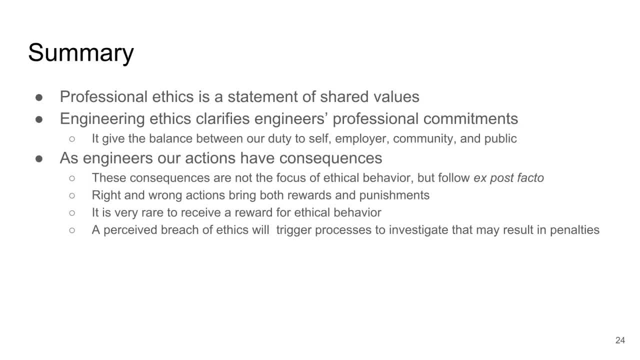 these ethics are are statements of shared values. they're they're not externally imposed. these are the values that good engineers have in common. we have these code of ethics that essentially help to clarify your commitments, and it helps you understand the balance between your duty to yourself, your employer, the community of engineers and and the public. as engineers, you have responsibilities.